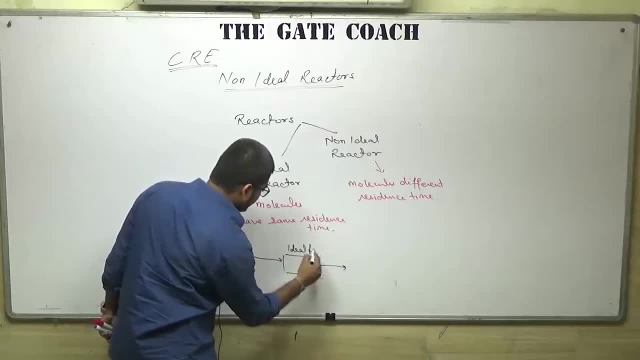 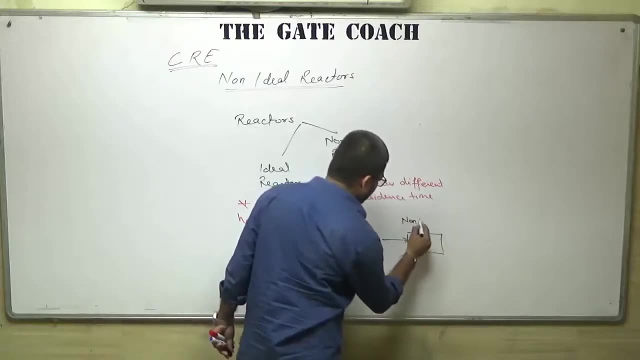 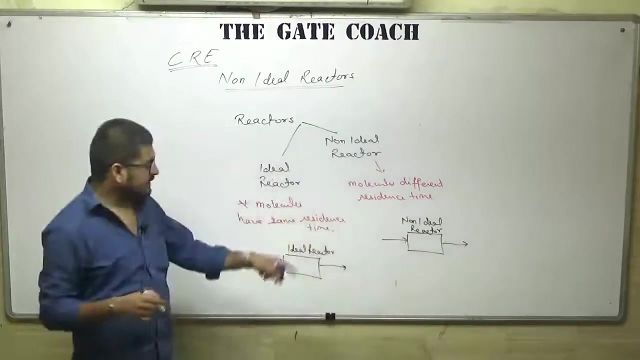 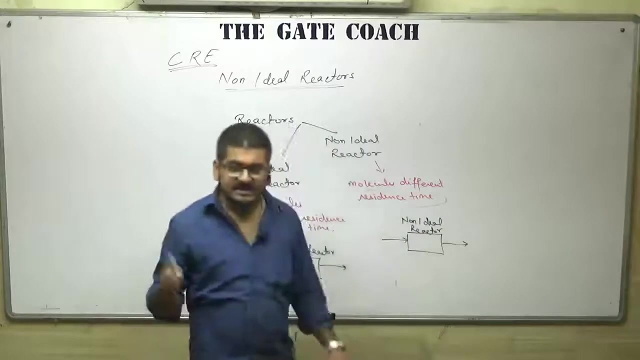 diagram of any ideal reactor: ideal reactor and this is a block diagram for a non-ideal reactor. molecules are going in, leaving, going in and leaving. and what is the residence time? so all of us know that the residence time is the time is spent by a molecule within the reactor. so, in case of 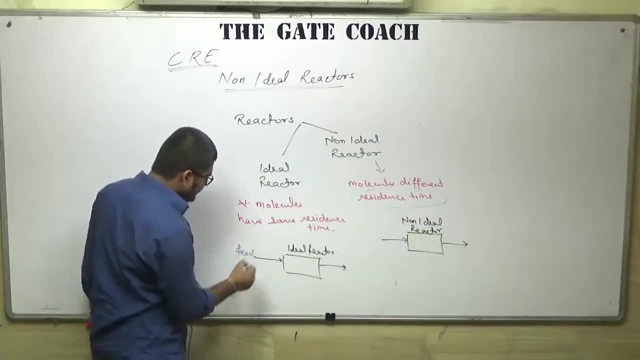 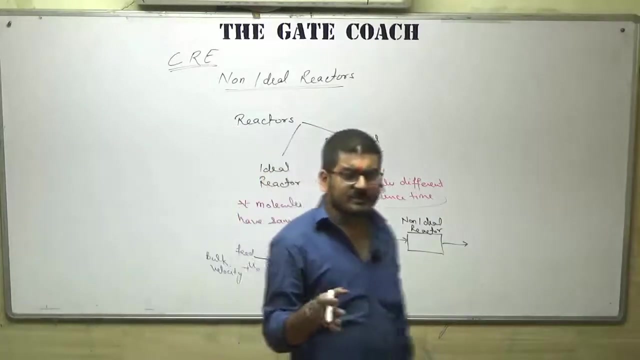 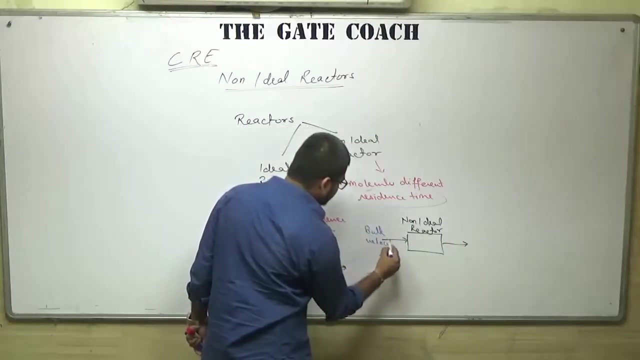 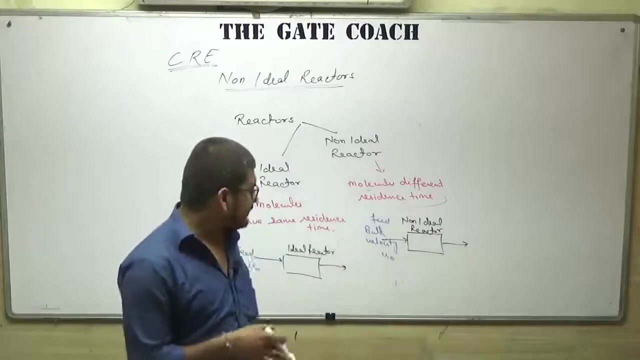 ideal reactor, we know that molecules are going in with some bulk velocity. let us say that is U0 or U0, and bulk velocity of all the molecules will be approximately same. in the same way here in non ideal reactor. velocity of feed, let's say you not, and that is that to- will be same for all the. 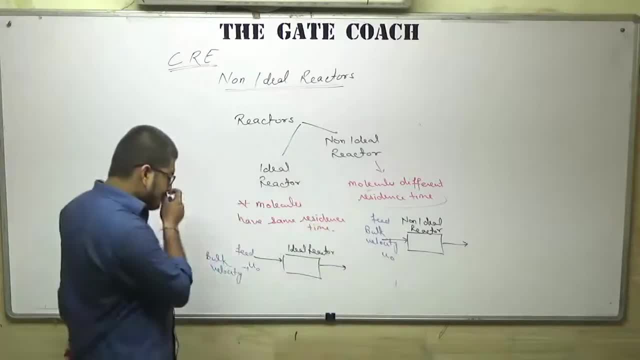 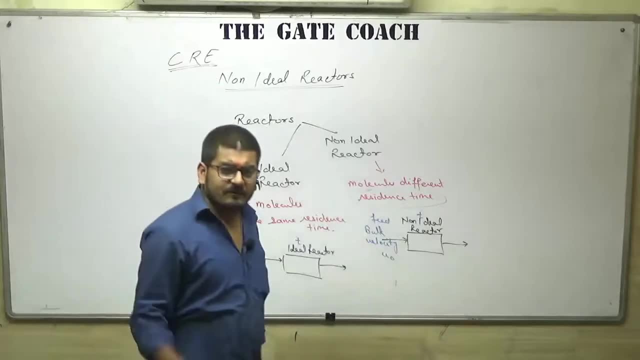 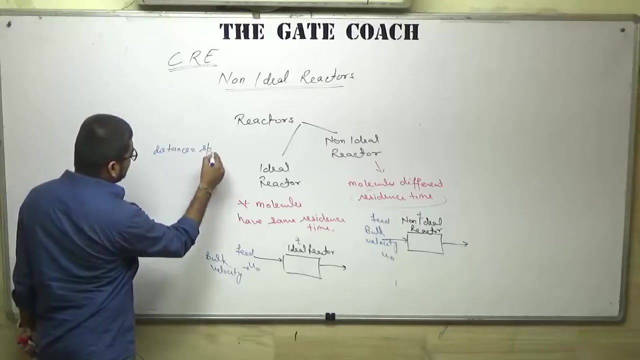 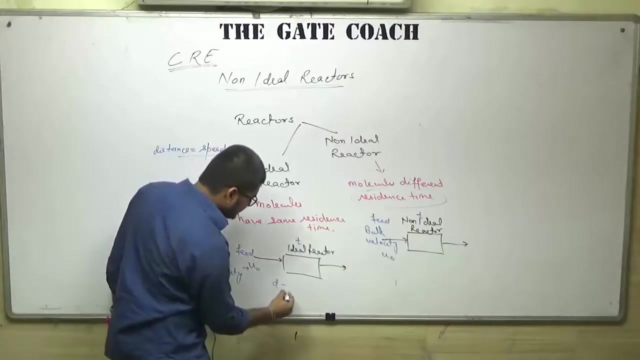 molecules approximately. okay, and this is the residence time T. so now all of us know that distance is equal to speed into time. so the same way here. distance traveled by molecule within the reactor will be the product off the bulk velocity of molecule and multiply by their resistance time. in the same way, 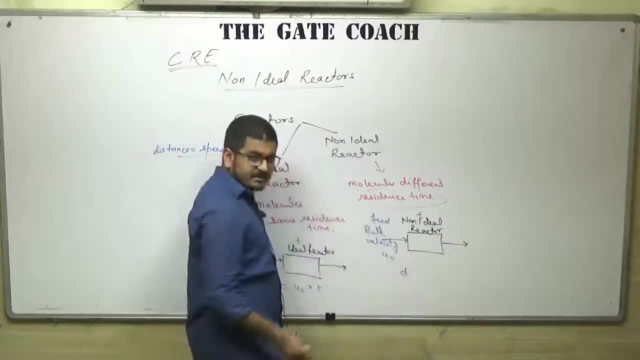 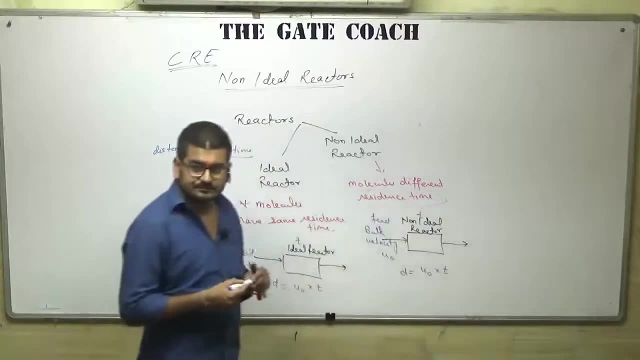 here the distance traveled by the molecule within the reactor will be equal to the, the, the bulk velocity of molecule and the residence time of the molecules. so now you can see that in case of ideal reactor, bulk velocity same and residence time is also same. so the distance 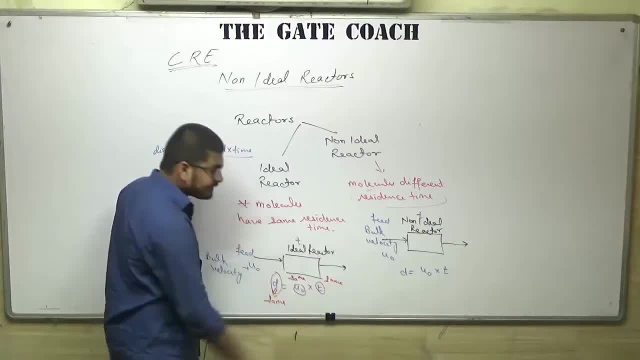 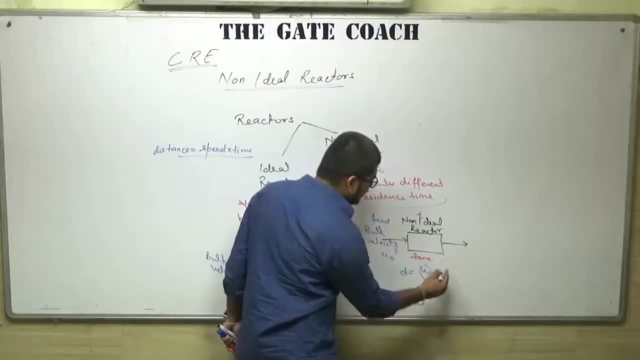 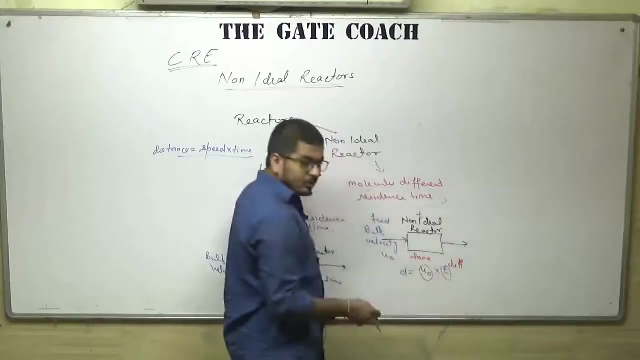 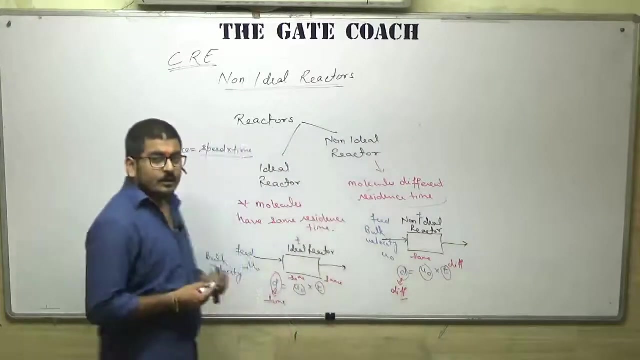 travelled by all molecules will be same as well. okay, but in case of non ideal reactor, bulk velocity of all the molecules is same, but the residence time spend by the molecule within the reactor will be different. so the product means the distance travelled by the molecule- will be different as well. so what is the meaning of that thing that in ideal 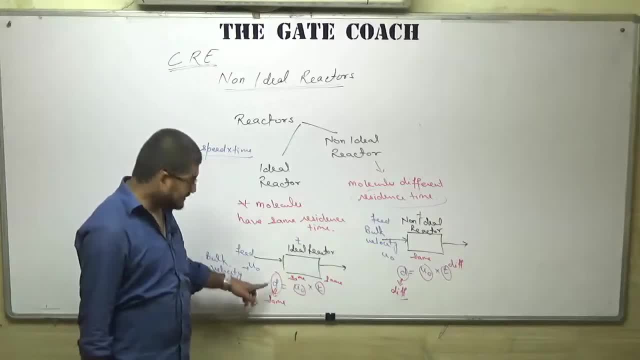 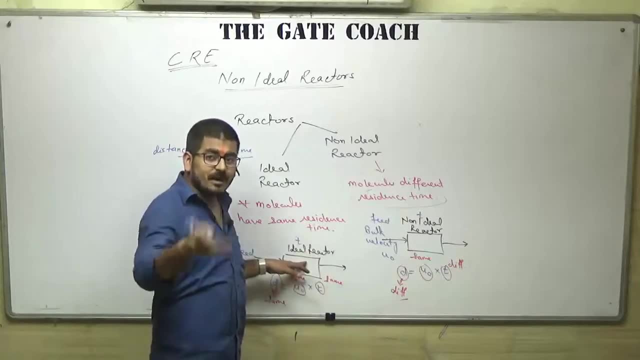 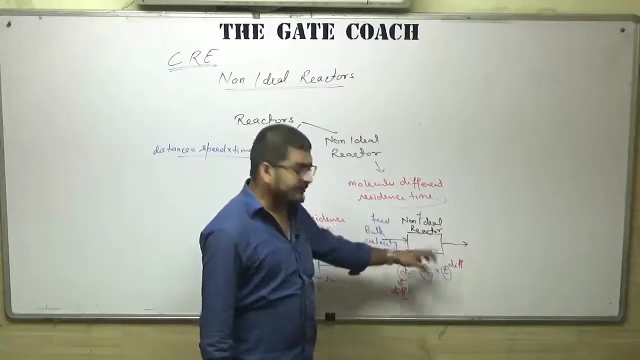 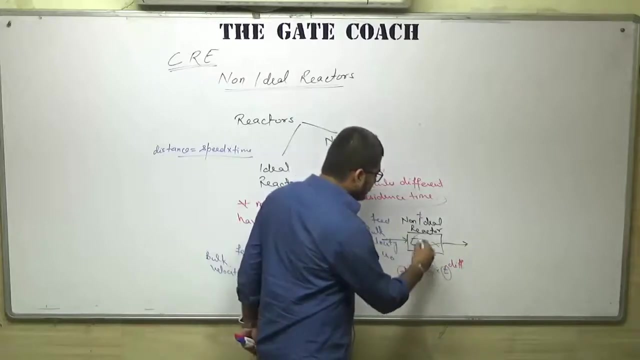 reactor all molecules travelling the same distance. okay, it means all molecules have same flow path, but in case of non-ideal reactor, distance travelled by all molecule is different. so it means we can say the flow path for all molecules is different in case of non-ideal reactor. 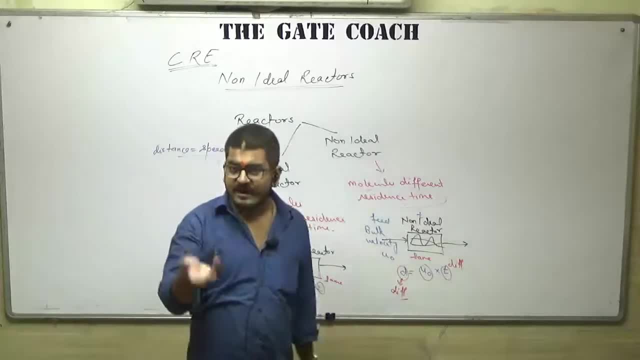 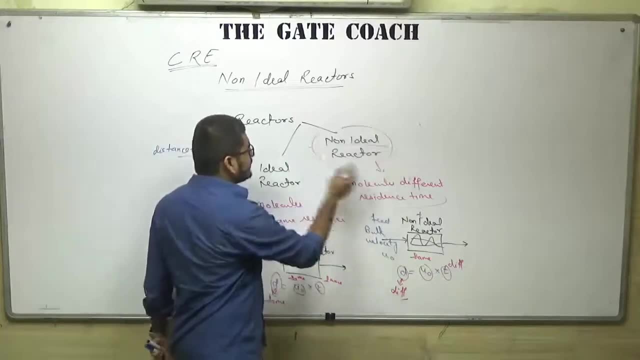 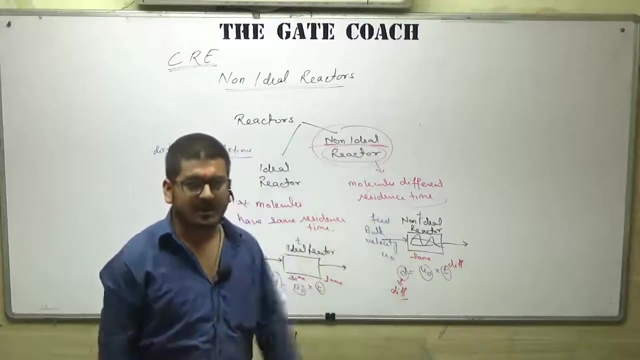 and flow path is provided by the reactor. that depends on the reactor geometry. that's why we use the term non-ideal. reactor means this non-ideality is basically the characteristic of reactor, not the reaction mixture or anything else. I think it is clear to all of you. why the residence time in non-ideal reactor is different for different molecules. because the distance travelled by molecules, the flow path of the molecules in the reactor is different and that depends on the reactor geometry. so that is something about the non-ideality of reactor. now, 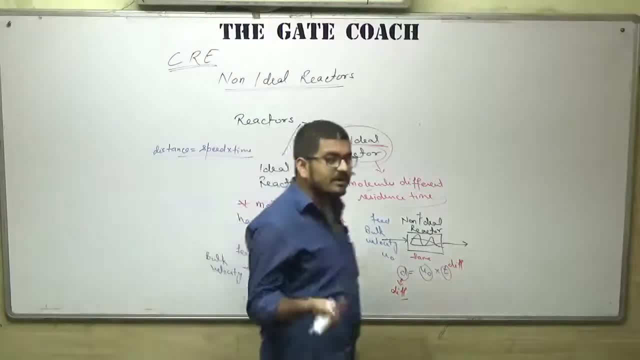 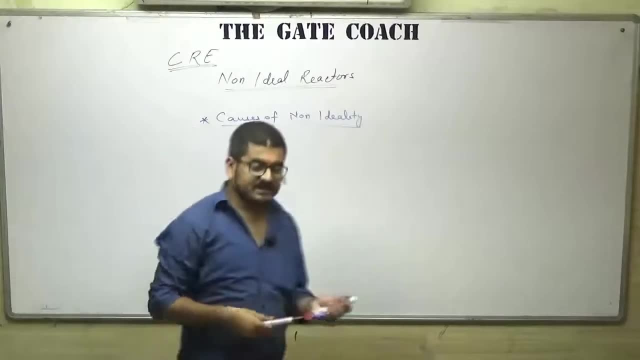 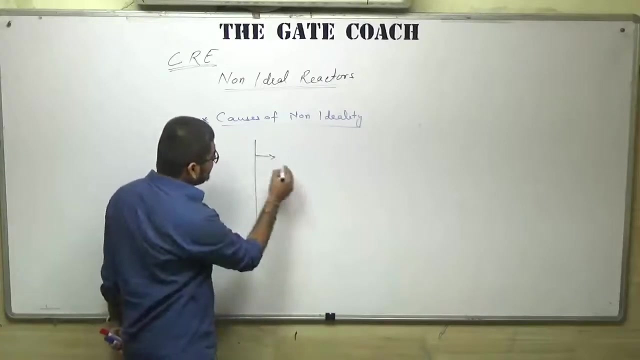 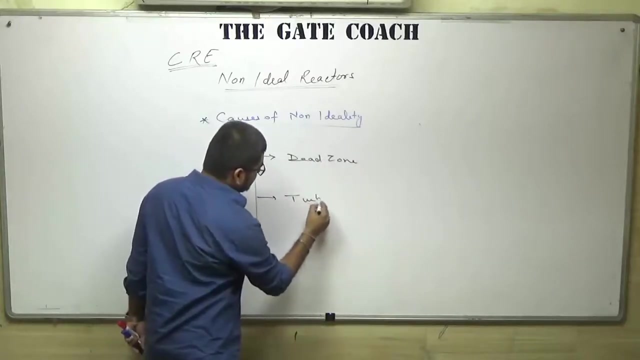 now we will talk about the causes of non-ideality, why the molecules have different residence time here. so basically there are n number of reasons for non-ideality, but here we will talk about mainly three. one is dead zone, second one is turbulence and third one is bypass zone. 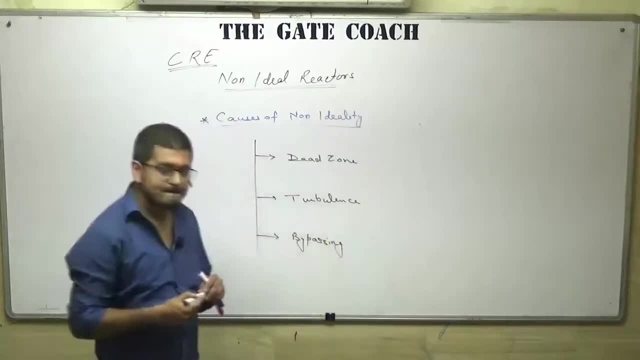 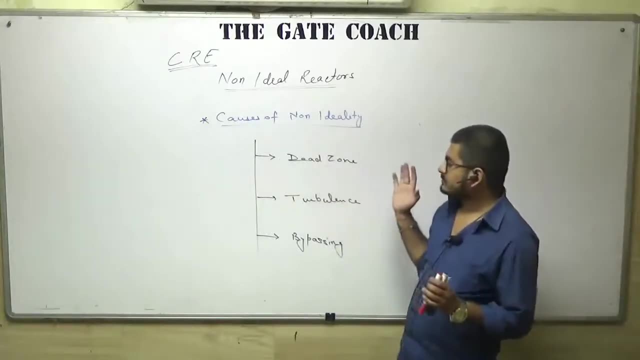 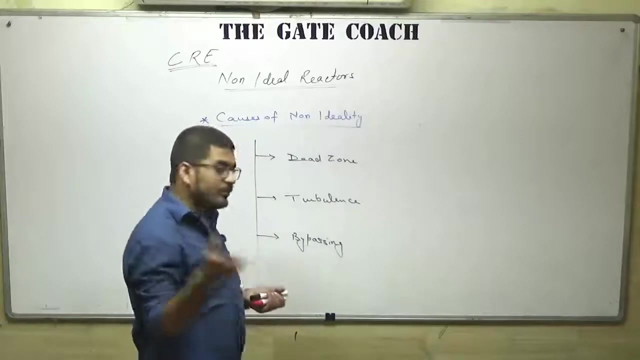 so what is dead zone? as the name suggests, dead zone, as it happens in life. if a person is dead, then the probability of that person to come back in real life is almost zero. or we can say he may come back in real life after infinite time. so in the same way, 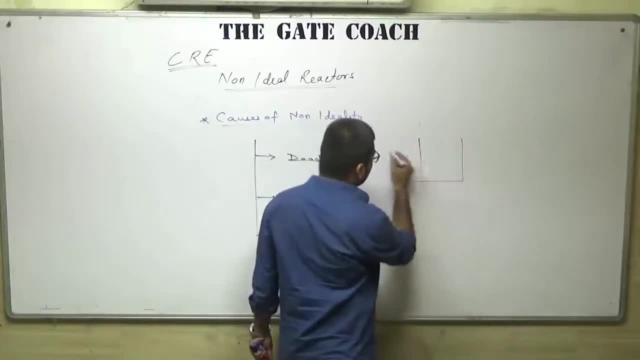 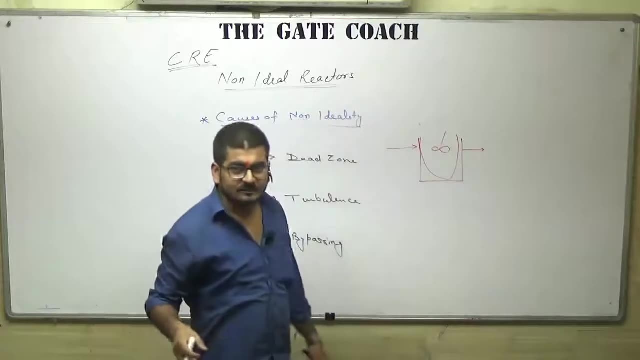 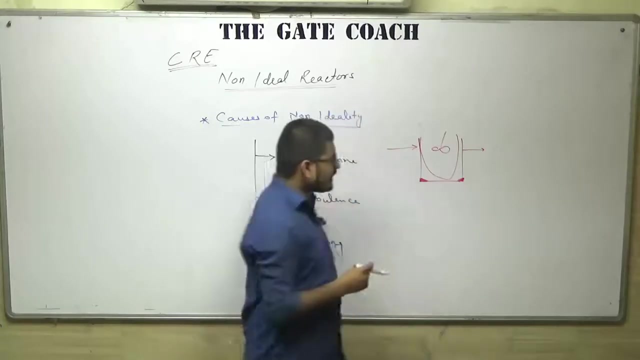 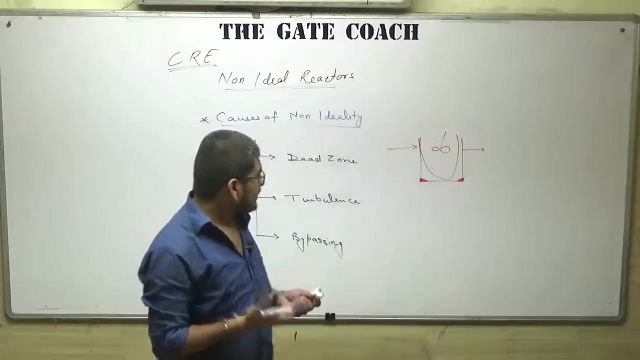 in a reactor where we have extreme corners. this is inlet, this is outlet, and we know that normally the mixture profile is parabolic because of the agitation. so, because of these extreme corners, if any molecule got trapped in these, then the probability of those molecules to leave the reactor will be almost zero. 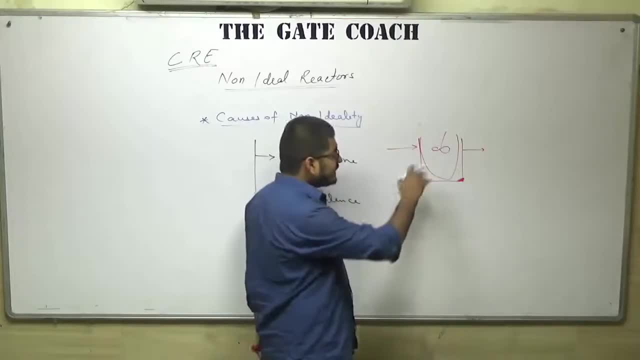 and the time spent by these molecules will be almost zero. and the time spent by these molecules will be almost zero, and the time spent by these molecules when they are not leaving the reactor, then obviously the time spent by the molecule in the reactor, the residence time, will be infinite. 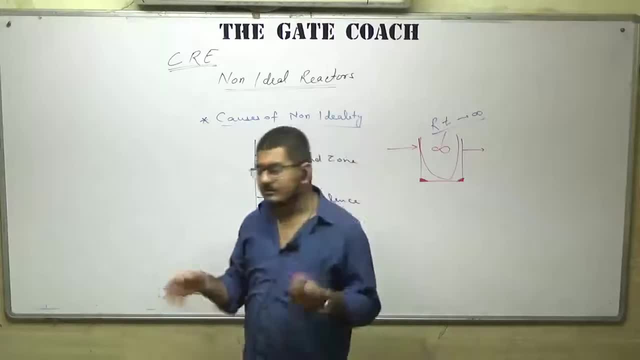 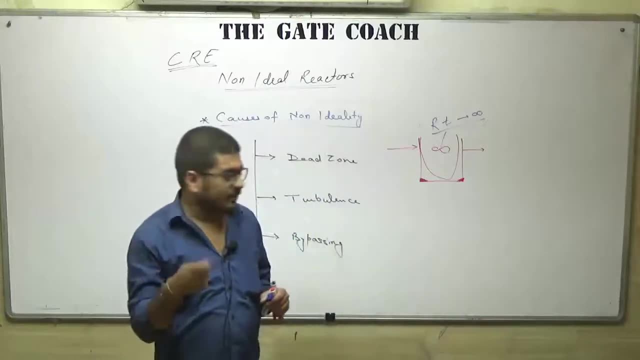 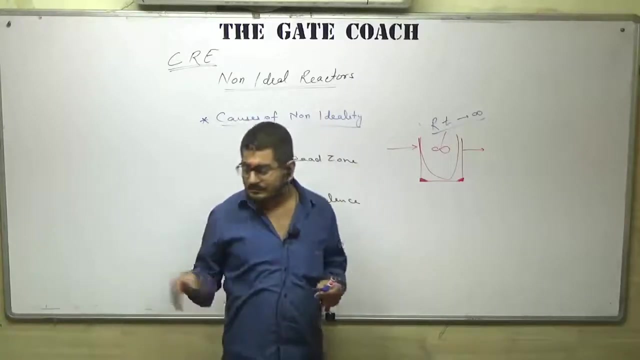 it is just like if we see in our daily life, if we have a house and we clean the house. so if there is an extreme corner, try to remove the dust with the help of a broom or anything, any cloth, then it will not come, do you understand? 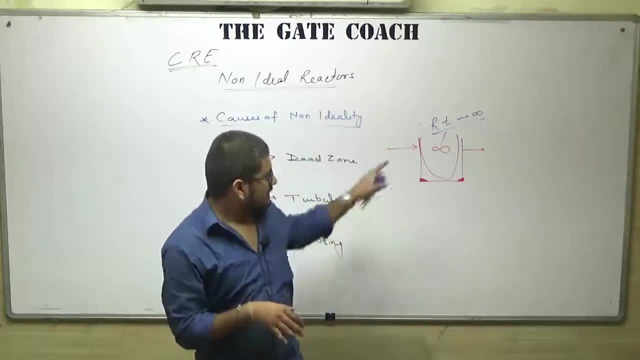 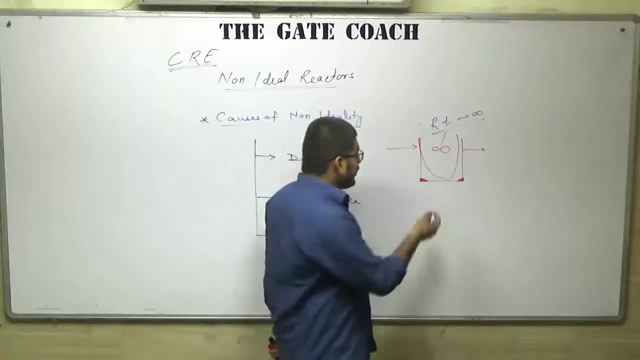 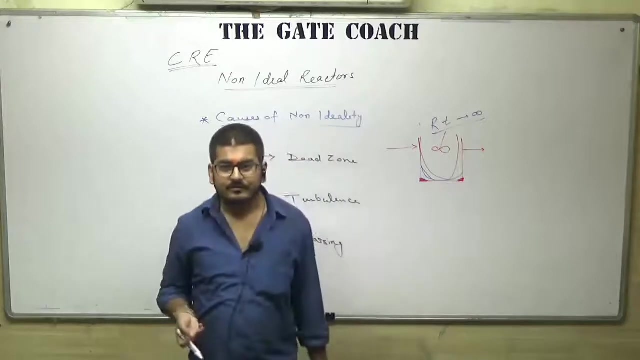 it will not come without vacuum cleaner. so in the same way, if any molecule gets trapped here, then it will not come out, and that is the reason maybe nowadays, the modern age reactors have hemispherical or cylindrical bottom to avoid the extreme corners, so that we don't have 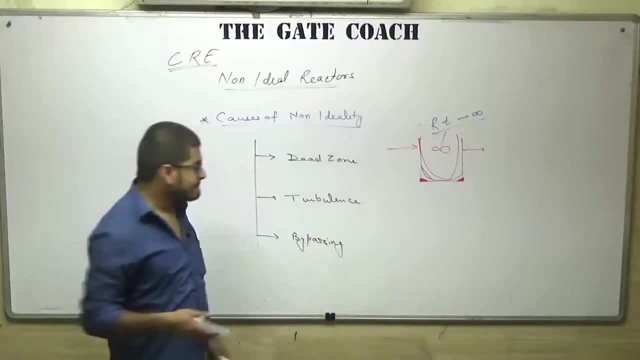 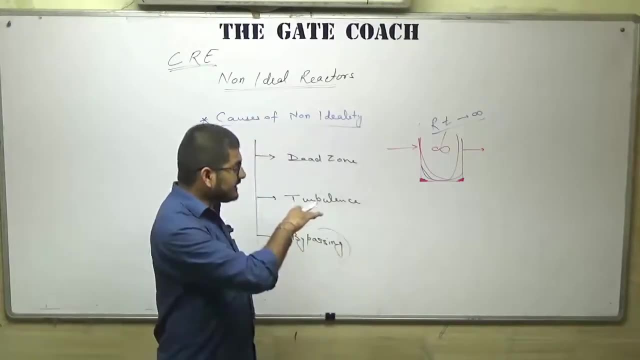 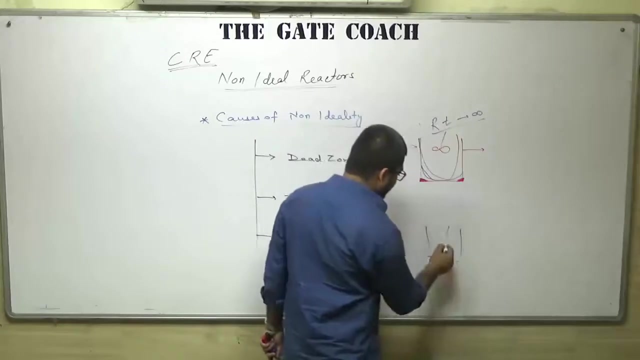 the problem of that zone. ok. and next one is bypassing what is bypassing? to skip the process when some amount of inlet is directly sent to the outlet, by skipping the process in the same way, here in this reactor, this is inlet, this is outlet. ok, logically. 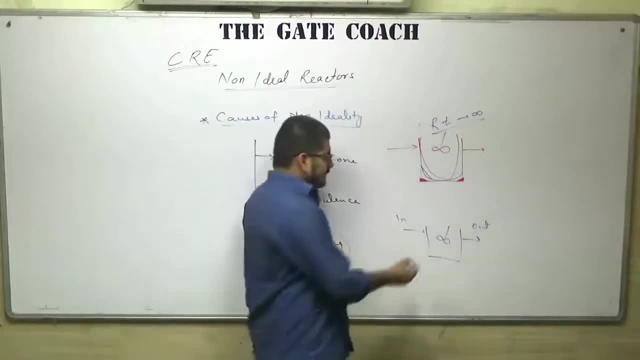 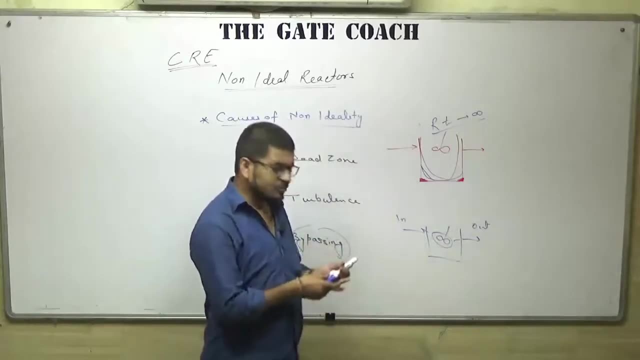 if the molecule is going in the reactor, it should get mixed and then leave. that is the path the molecule should follow. but what happens in practical life? there are some molecules which directly go to the outlet. either they have very high velocity or they are not going to the outlet. 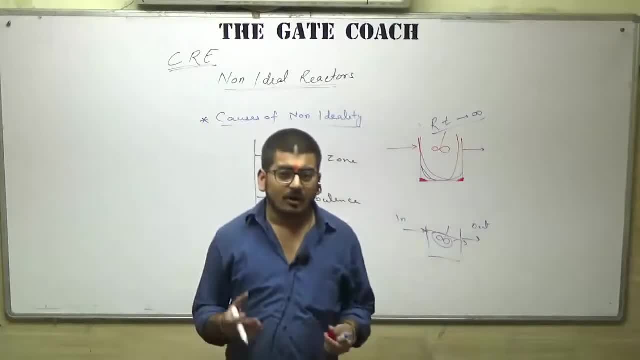 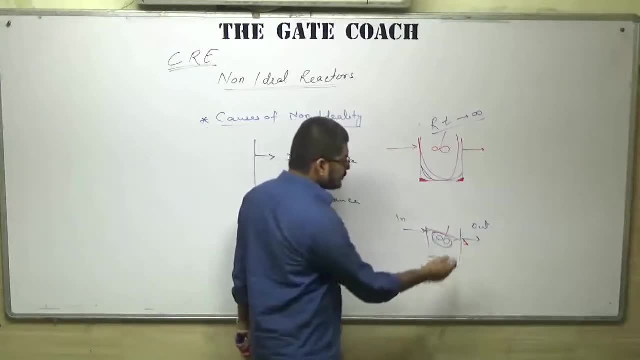 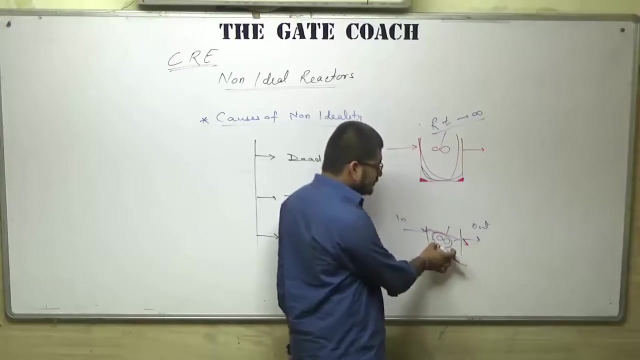 so the process is like. the process is like high velocity or very high inertia force, so they directly move to the outlet and skip this mixing zone. so we say that molecules are skipping the mixing, skipping this zone so means they are bypassing, and in this case you can see: 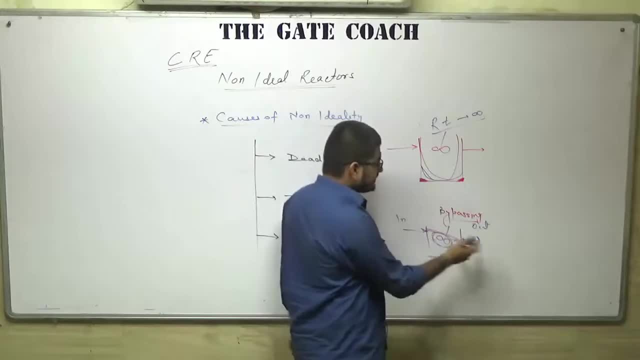 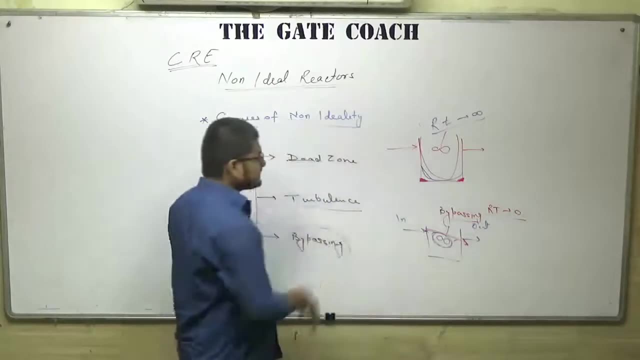 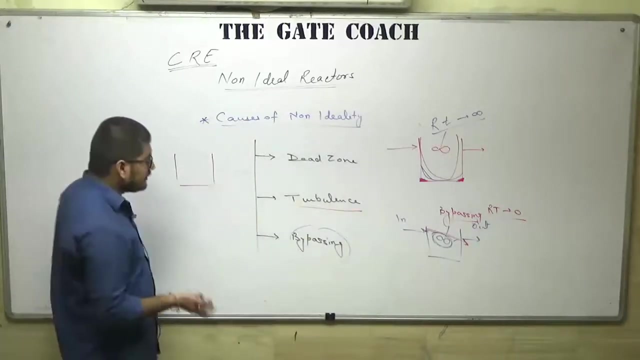 the residence time of the molecule in this reactor is very small, means almost zero or short residence time, you can say. next one is turbulence. what is turbulence? basically, it is related to mixing. ok, this is inlet, this is outlet, this is agitator, and you know that there is a mixing zone. 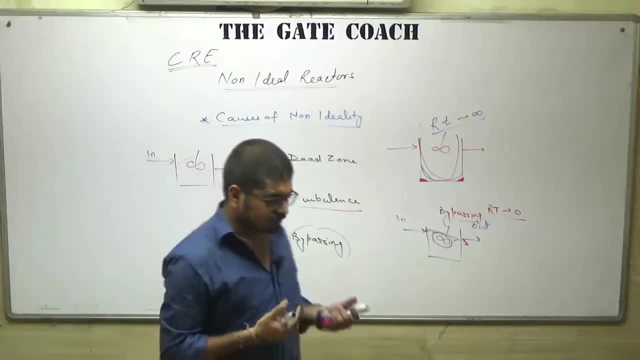 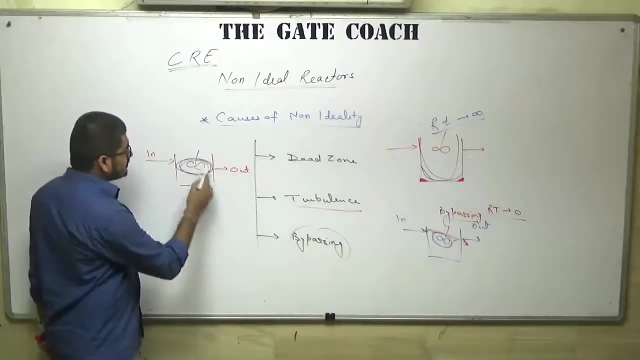 may be. you have heard about the term vortex formation and all ok. so you know that vortex formation is what, that there are some molecules got trapped in the mixing zone, some molecules get trapped in some vortex and it keeps rotating in it continuously, following the same path, and because of that, 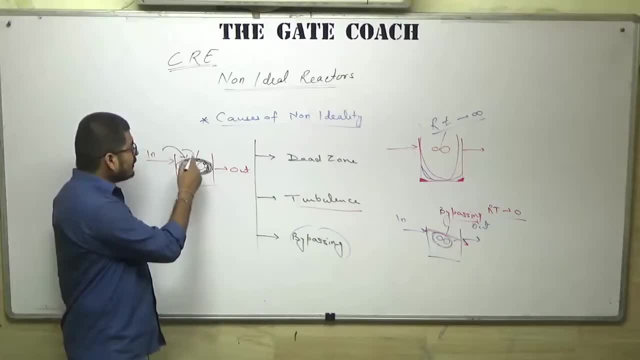 if there is any new molecule, it will not enter in the mixing zone because there is no vacant space and, in the same way, if any molecule is trapped in this, it will take a very long time, very large time, to leave the reactor. ok, that's why, in case of turbulence, 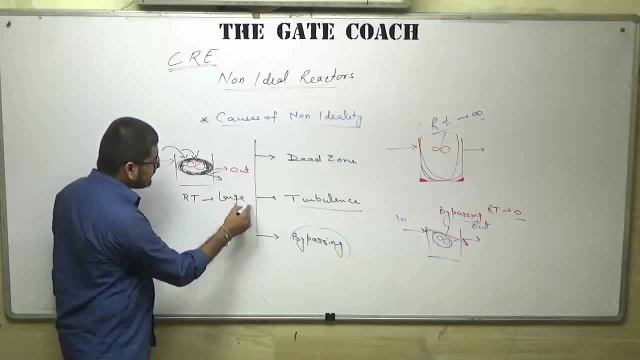 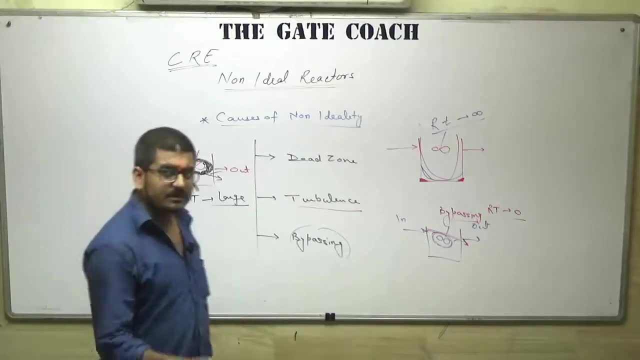 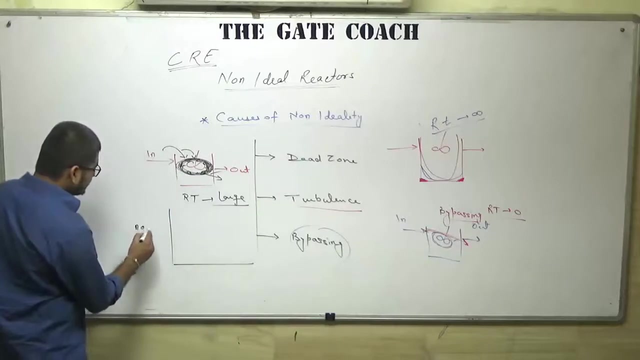 the residence time is very large- not infinite- because it is a part of process, so it definitely the molecule will leave the reactor, but after very long time. so if you draw a curve between number of molecules leaving the reactor to the residence time, then because of the bypassing, 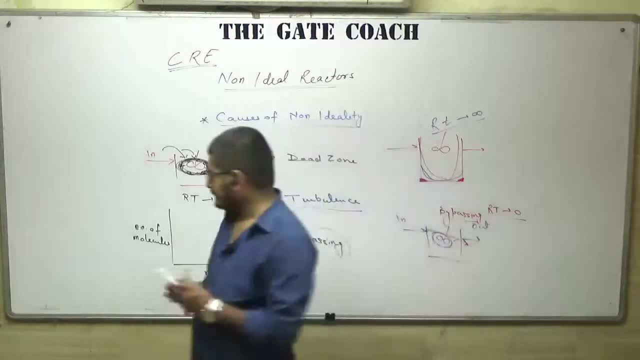 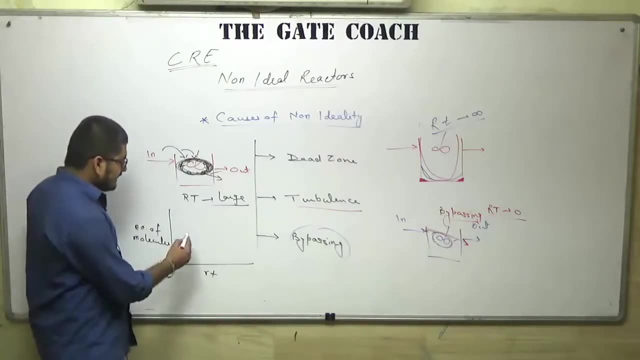 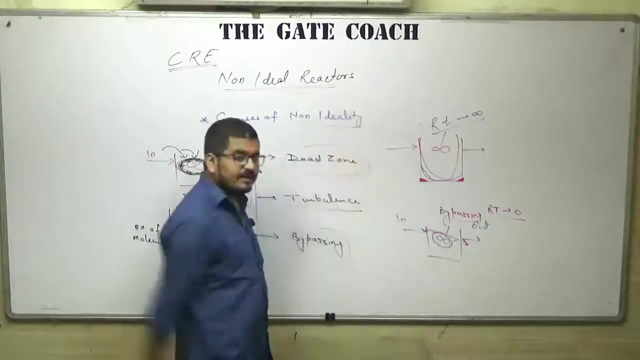 some molecules have very small residence time so they will leave early. then some molecule will leave the reactor near the mean residence time. then some molecules will leave because of turbulence, having have very large residence time, and if there is any molecule in that zone which has infinite residence time, 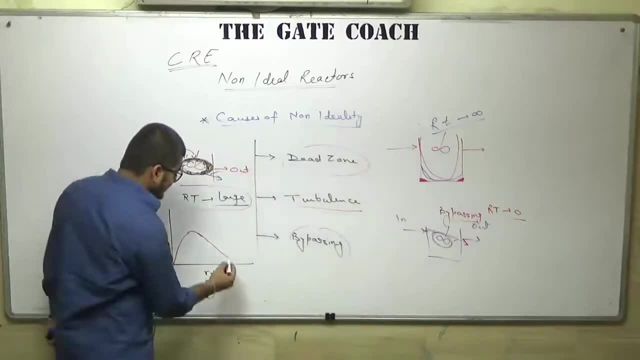 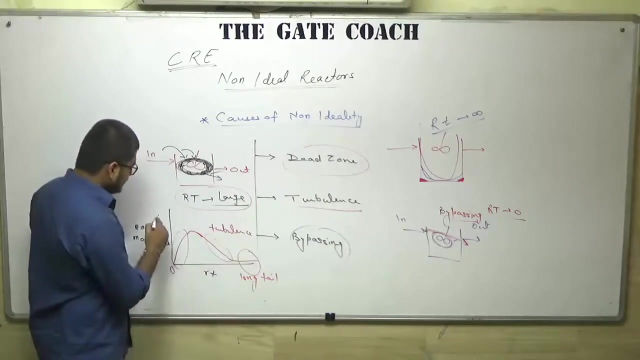 or very, very large residence time, so that molecule will not leave the reactor. so that's why this curve will never going to touch the x axis, ok, and this long tail represents the dead zone in the reactor. this is turbulence and this is bypassing. ok, very short residence time. 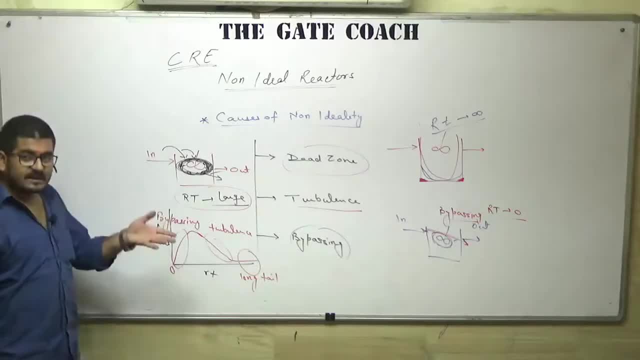 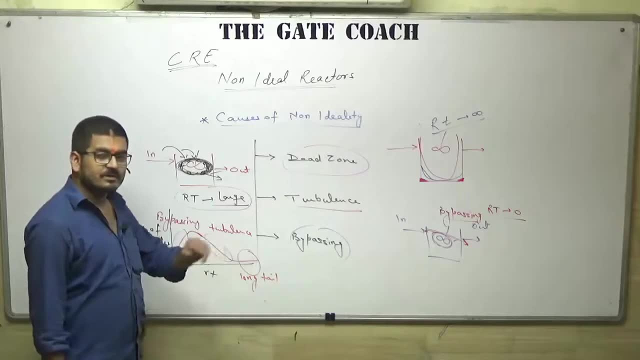 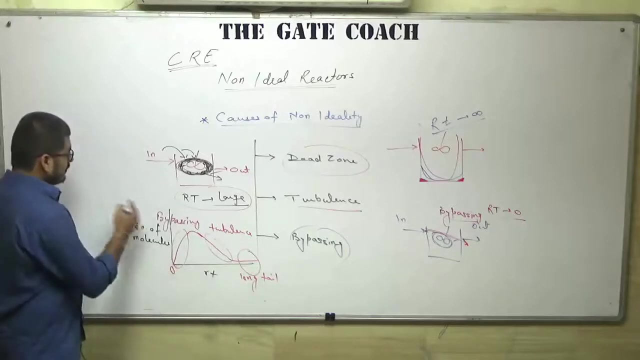 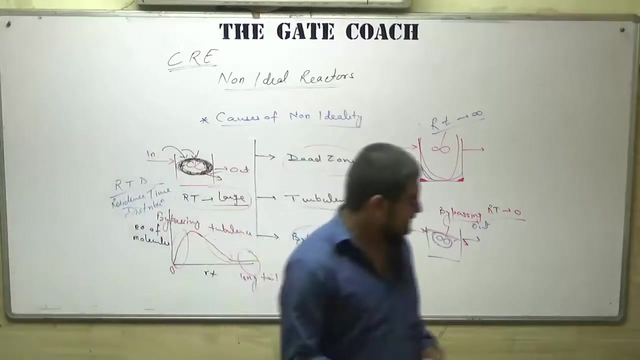 and we can see that in non ideal reactor molecules have different residence time. so when we draw the curve it is like a distribution curve and the analysis of this distribution curve of residence time of different molecules is known as RTD, that is, residence time distribution. ok, so this is something about basic part. 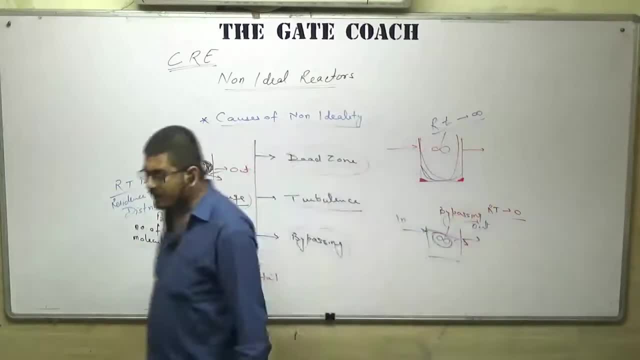 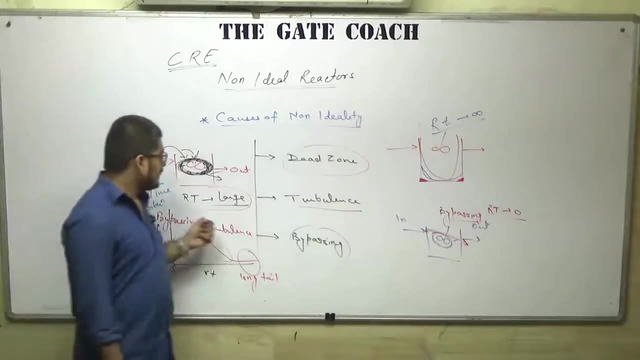 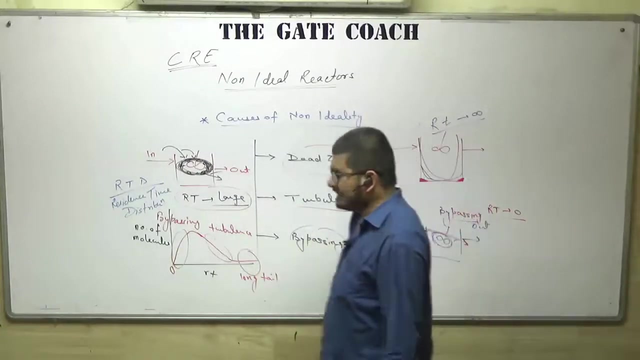 after that I will discuss about the how to find out the residence time distribution curve in the reactors and what is the parameter or what is the element we use to identify the residence time distribution curve- that is basically tracer- and how to inject that tracer in the reactor. 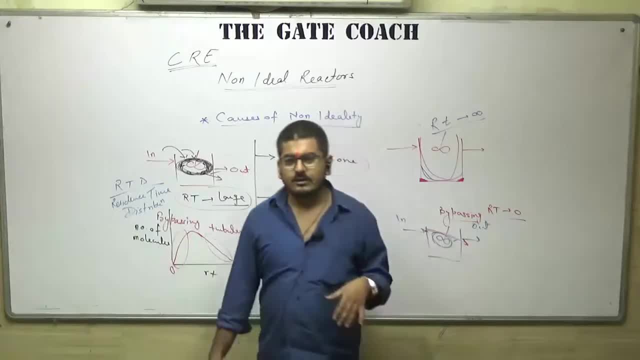 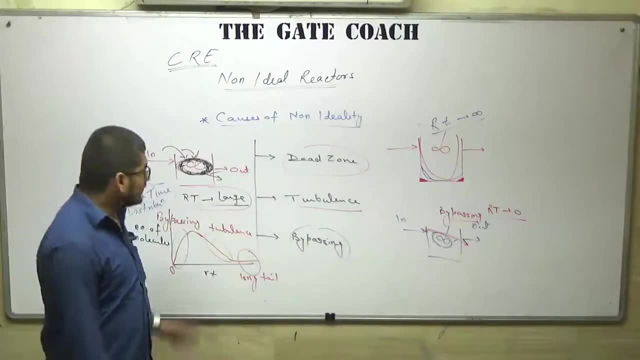 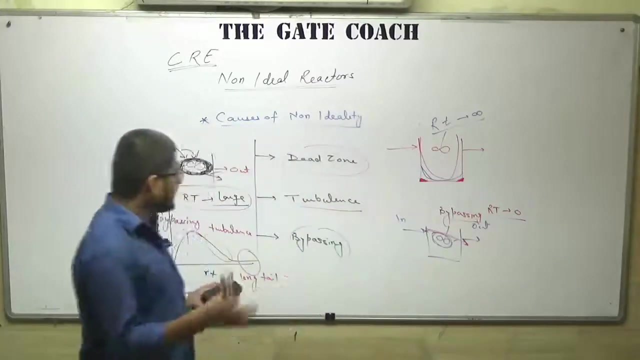 but that I am not going to discuss in this video. that we will discuss in the class or you can ask me personally. ok, so now I will directly move to the new topic, that, the input methods of tracer in the reactor. so first I will talk about the pulse input experiment. 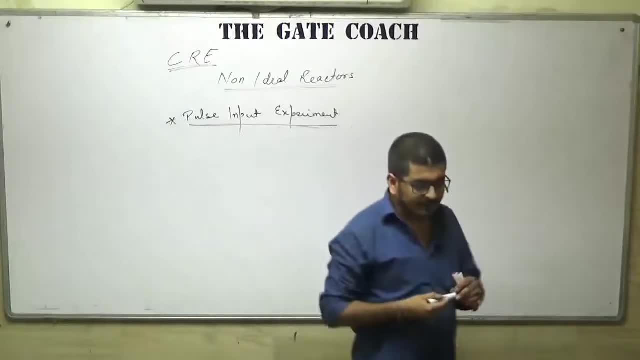 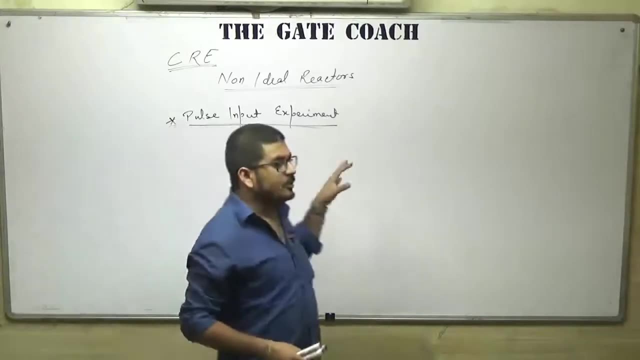 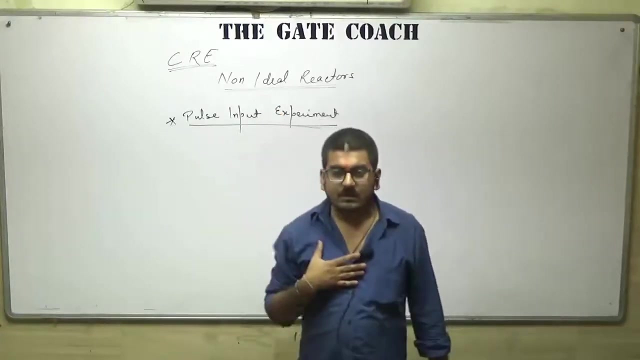 see, guys, as of my experience in this industry from last 5-6 years, this is one of the under rated topic of CRE because people think it is very difficult- the RTD part- but I tell you that this is the most easy topic of this subject. 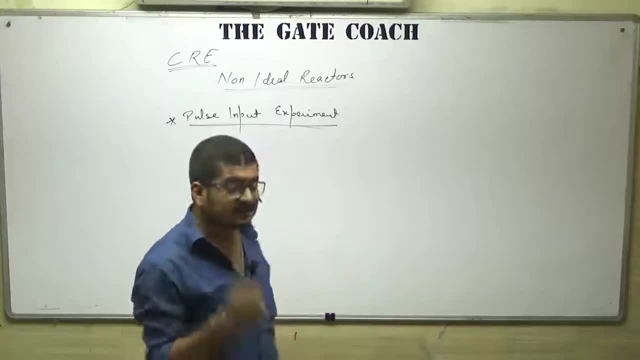 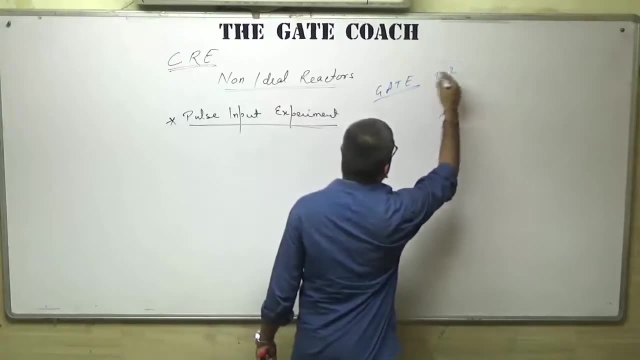 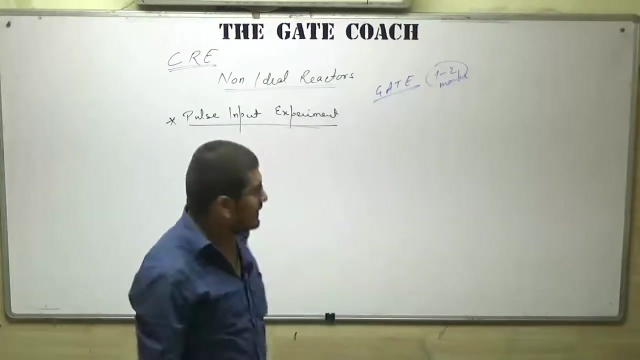 and you can score 100% marks from this topic, because every time in GATE exam you will get a question from this topic of 1 or 2 marks. ok, I don't know why this year there was no question on this topic, but before that, from 2000 to 2017. 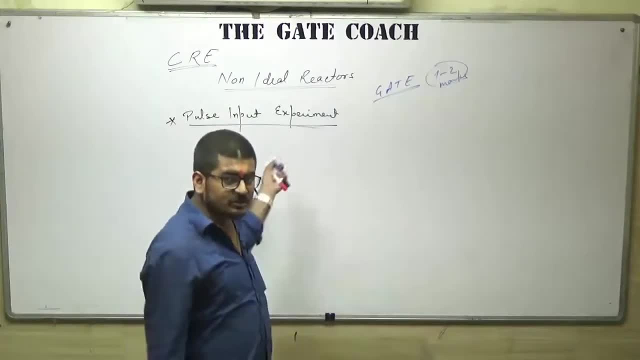 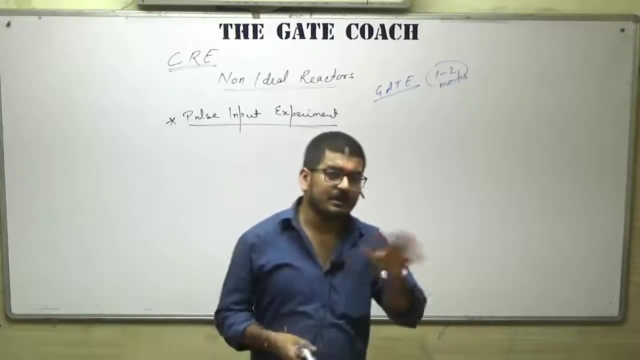 we were having a 1 or 2 question from this topic every time in the exam and those are very basic and easy question. so if you know the meaning of each and every term here and you know the basic mathematics of class 10th and 11th, 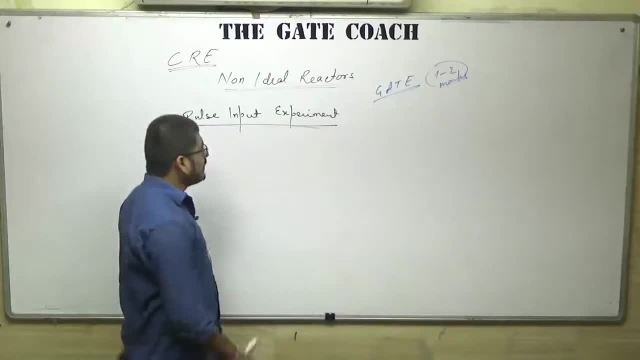 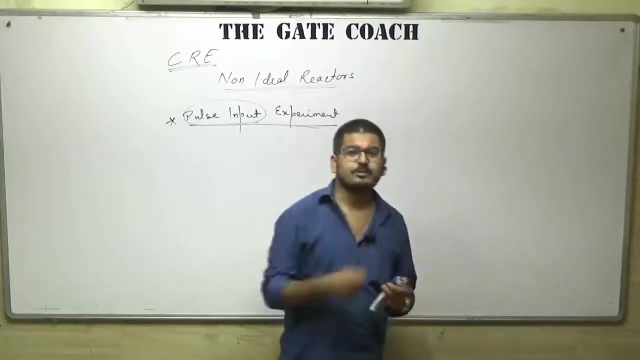 then you can solve any problem of RTD. ok, how that we will discuss. so pulse input experiment. one point is: what is pulse input? so we know that pulse input is basically the sudden injection, sudden disturbance in the input profile for a very small fraction of time. 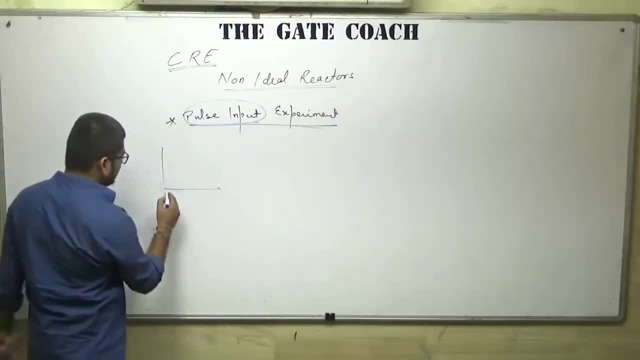 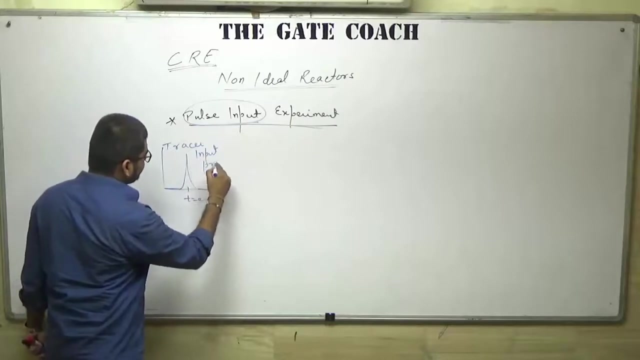 like this: there is nothing going on and suddenly there is a disturbance, and then again back to 0. so this is, let's say, at t, equal to 0. this is the tracer inject profile or input profile. we can say to the reactor: sudden pulse is there. 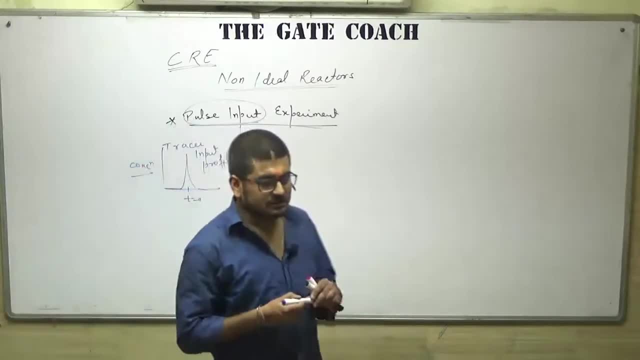 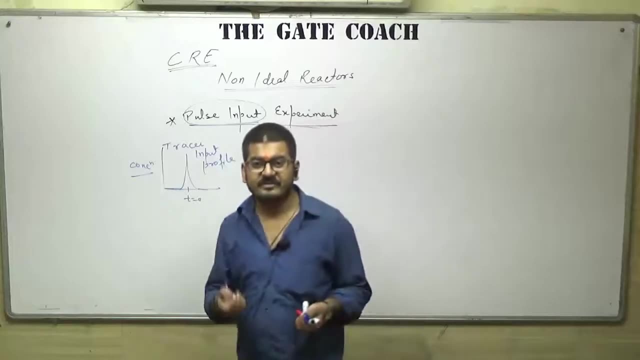 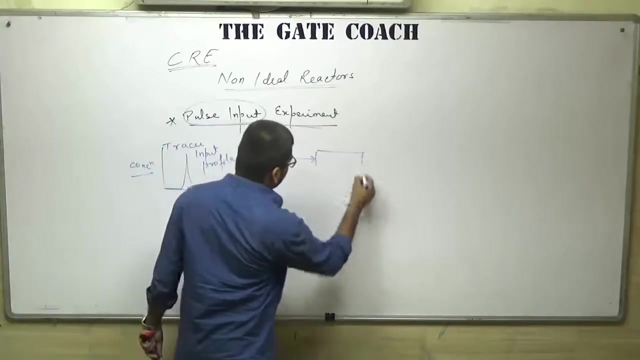 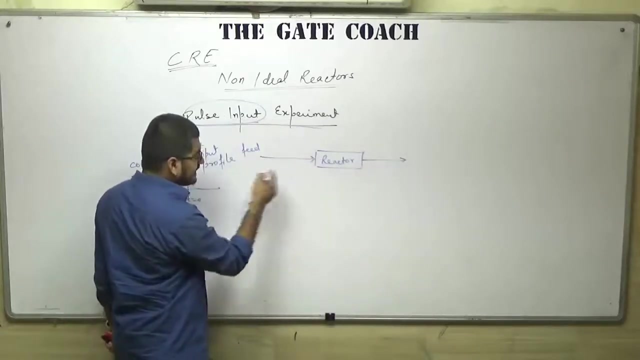 ok, this is pulse input, just like we use to have, we use to inject the serum or any medicine with the help of injection in any human body. ok, so let's say, if I draw a block diagram of any reactor, so this is the feed going in the reactor with the volumetric flow rate V0. 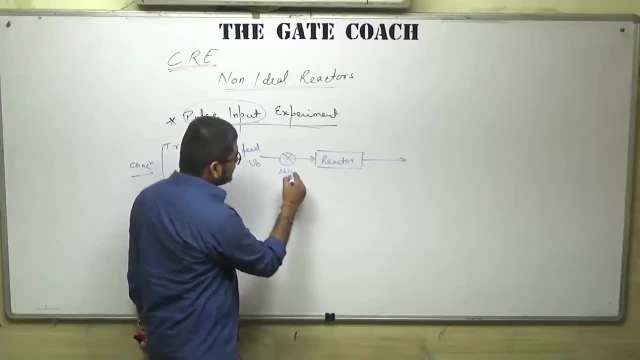 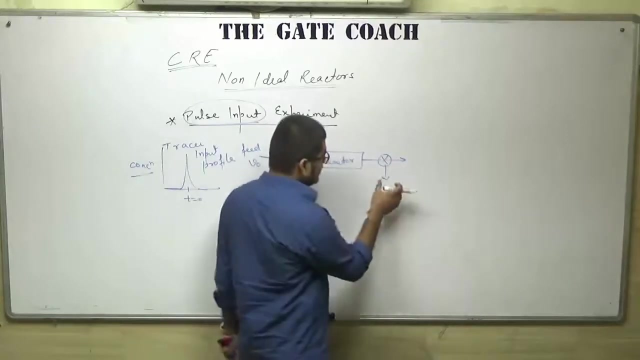 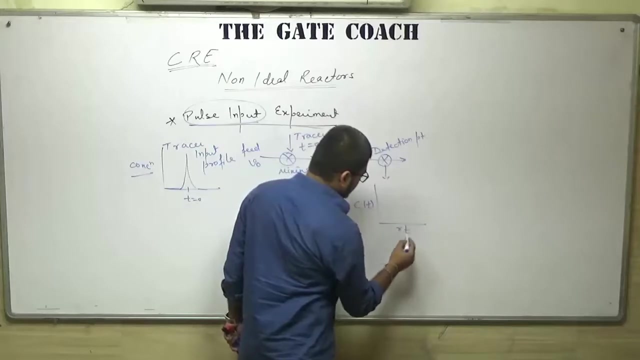 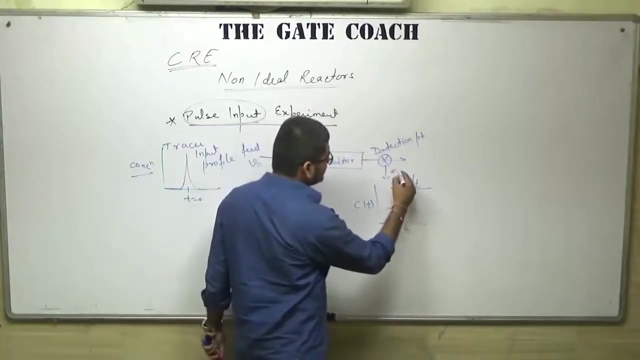 and this is the mixing point where I am injecting my tracer at t equal to 0 and at the reactor outlet. this is the detection point where I am measuring the concentration of tracer with time. ok, and this is the concentration of tracer. that is basically the exit concentration of tracer. 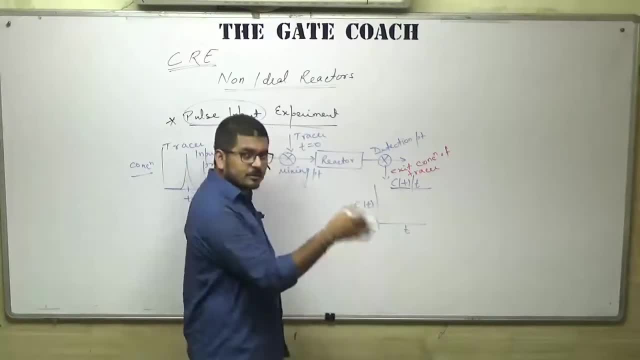 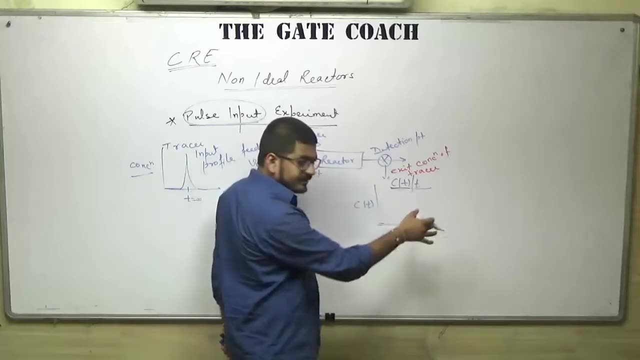 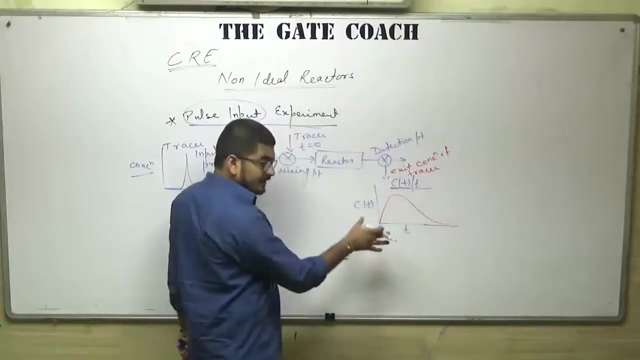 ok with time. so you know that because of the non-idealities, the exit concentration will be different for different time period. ok, and when you draw the curve, the curve will come something like this: and the curve drawn between exit concentration of tracer versus residence time for pulse input experiment: 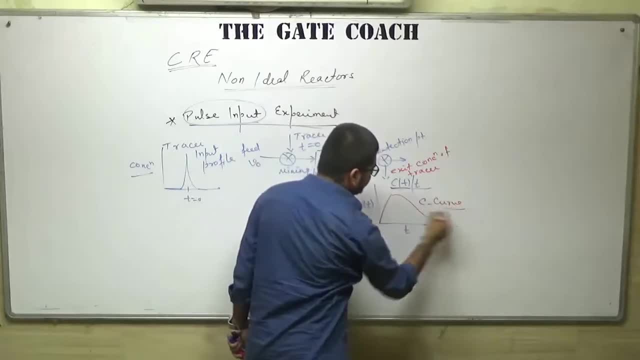 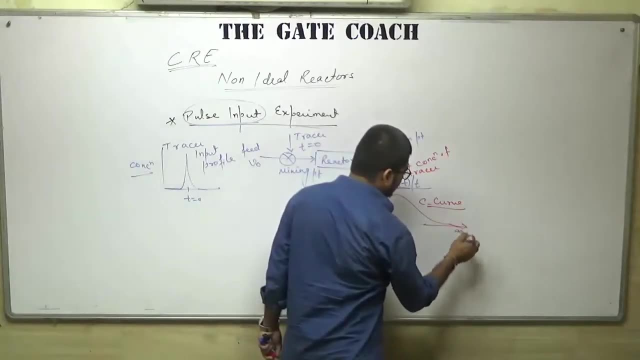 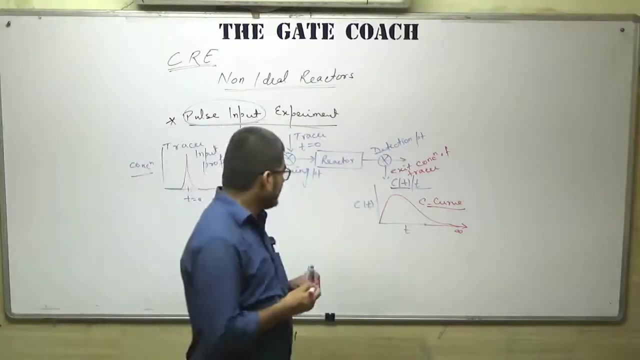 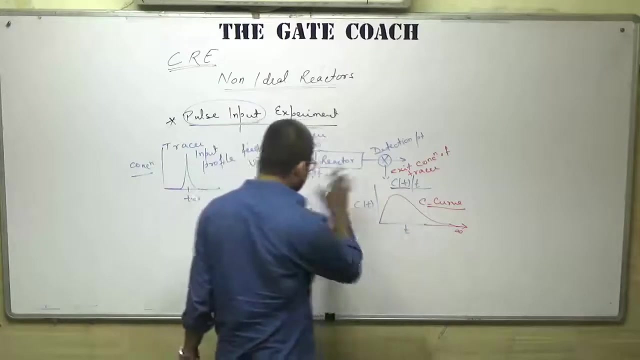 is known as C curve. ok, and at infinite time that curve will touch the x-axis means all molecules will leave the reactor. ok, so how to find out that curve and all that we will discuss next is: and all these things we can find out by with the help of material balance. 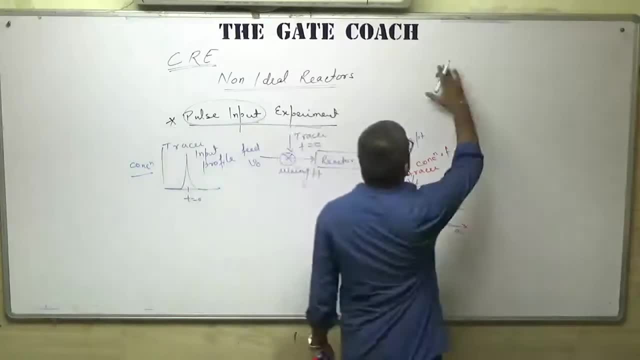 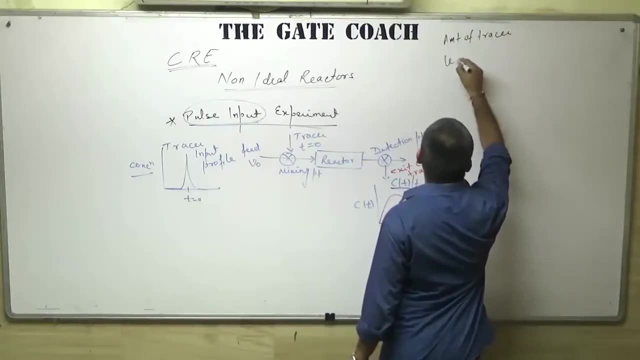 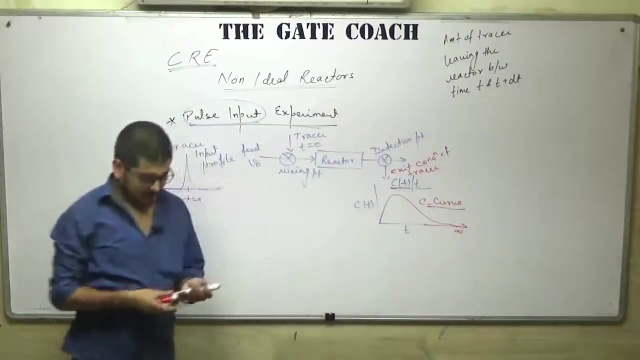 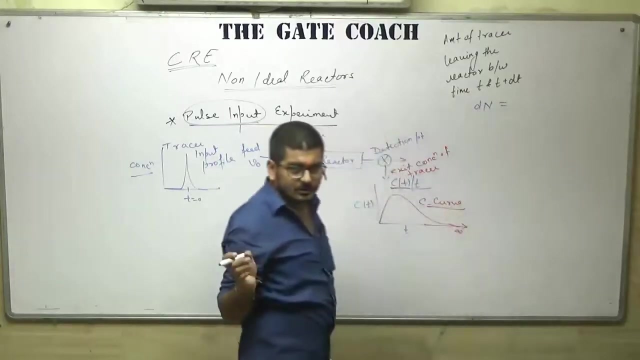 or mole balance over tracer. ok, so let's say we want to calculate the amount of tracer leaving the reactor between time t and t plus dt. ok, and that is, let's say, dn. n represents the number of molecules of tracer, so dn is the amount of tracer leaving the reactor. 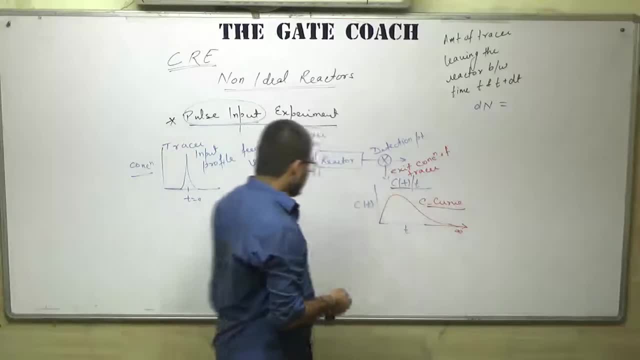 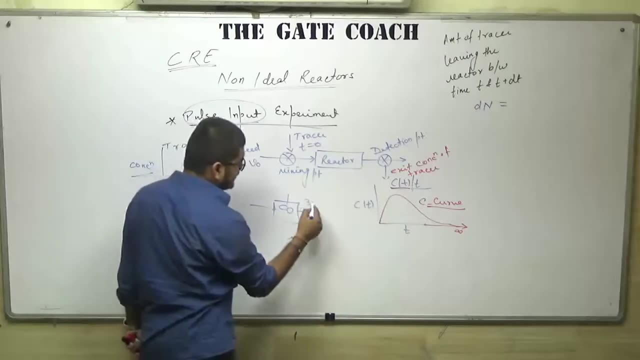 between time t and t plus dt. ok, now see, you know that if there is any tank and the exit flow, exit flow rate is, let's say, 3 kg per minute, ok, then how much amount of this fluid material will leave in 3 minutes? that is, 3 into 3. 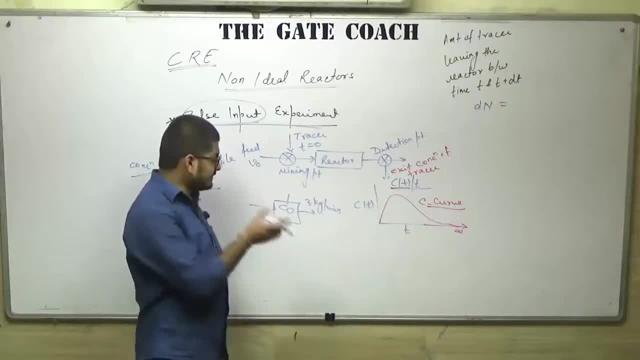 9 kg and how much amount of this material will leave between 3 minutes and 4 minutes, that is 3 into 4, 12 minus 3 into 3, 9, that is 3 kg. so in the same way, the amount of tracer leaving the reactor. 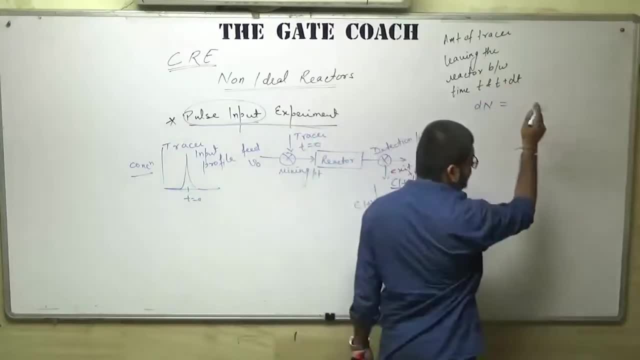 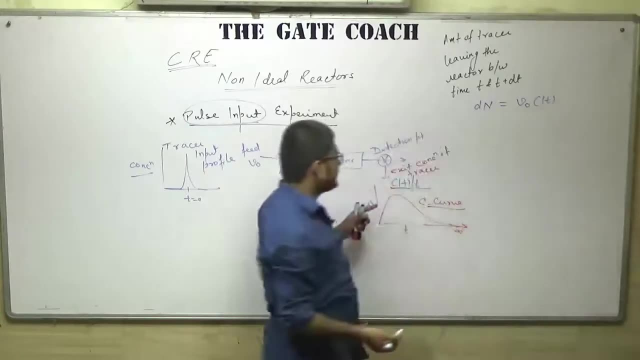 between time. t and t plus dt is the molar flow rate of the tracer at exit. that is the volumetric flow rate multiplied by exit concentration of tracer. so it is molar flow rate of tracer at exit. and this is reactor is operating at steady state. 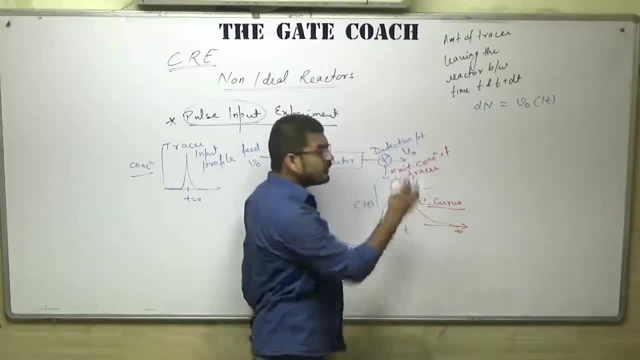 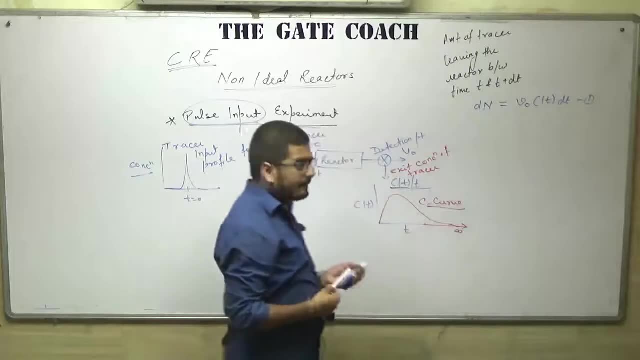 so that's why the outlet volumetric flow rate is will be v0 as well. ok, multiplied by the time interval, let's say equation 1, ok, so this is the amount of tracer leaving the reactor between time t and t plus dt. and let's say, if we divide this: 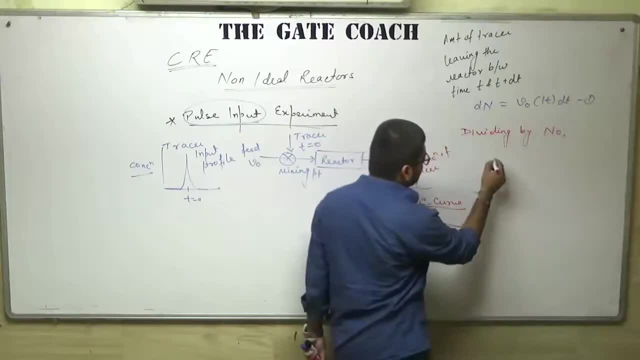 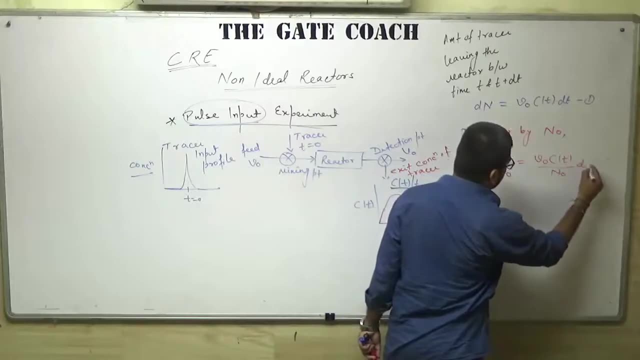 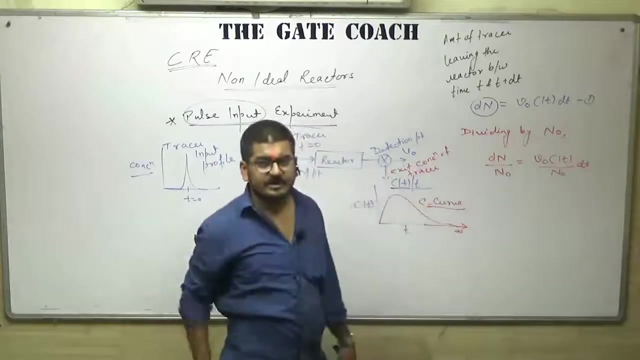 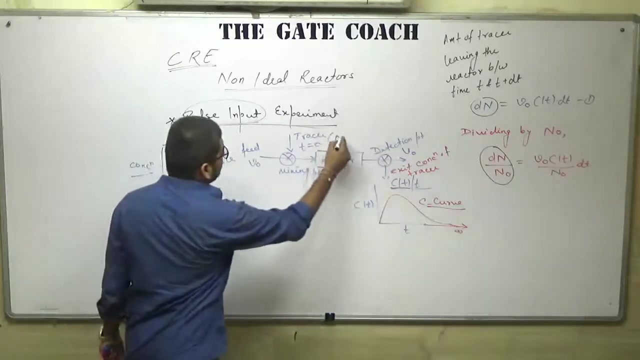 and by n0. that will be like: dn over n0 is equal to, and dn is the amount of tracer leaving the reactor between time t and t plus dt. so dn over n0, n0, which is the total amount of tracer we injected in reactor. so amount leaving the reactor. 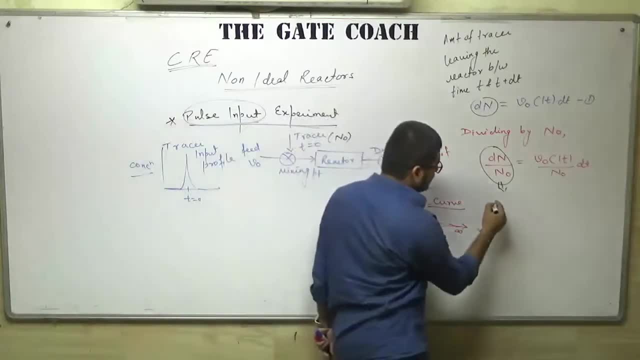 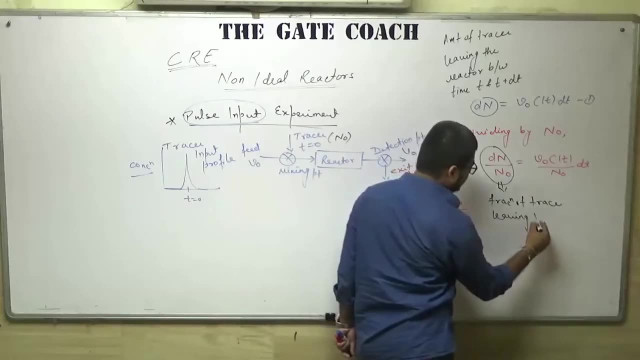 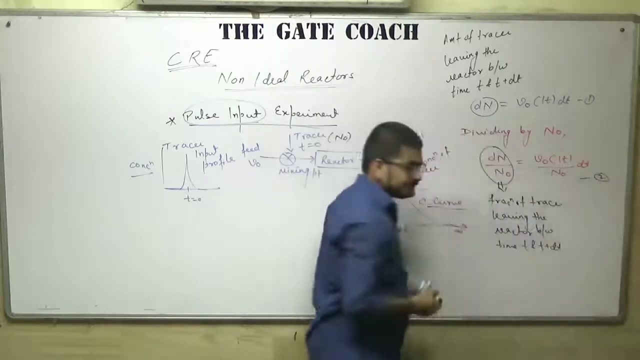 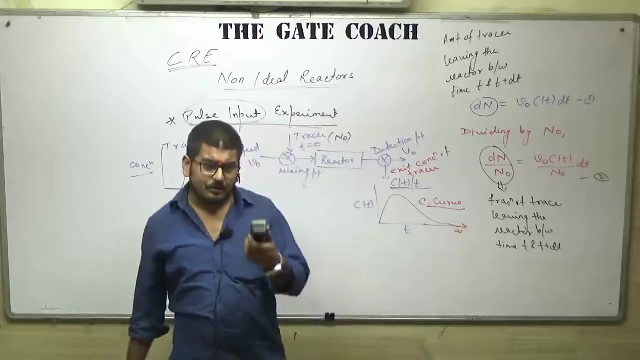 divided by total amount will be what fraction of tracer leaving the reactor leaving the reactor between time t and t plus dt, let's say equation 2. ok, and I believe that in statistical mathematics you have studied about the probability distribution, binomial distribution, Poisson distribution and normal distribution. 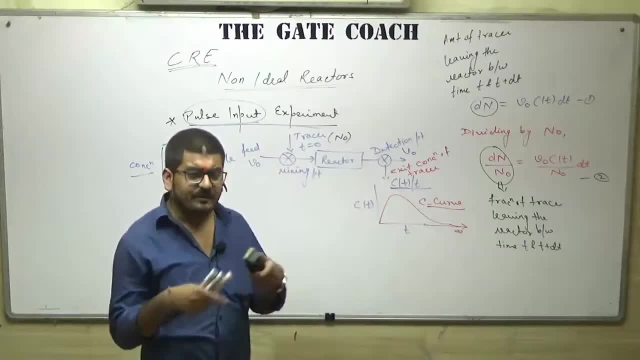 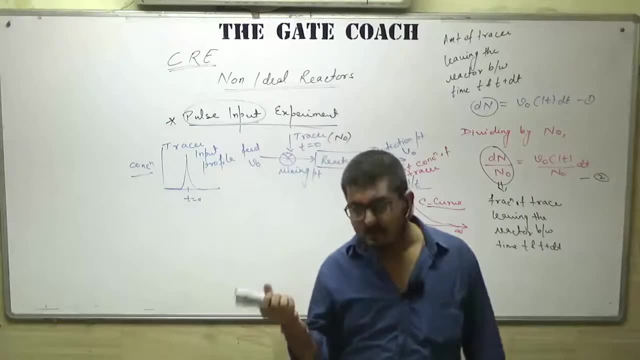 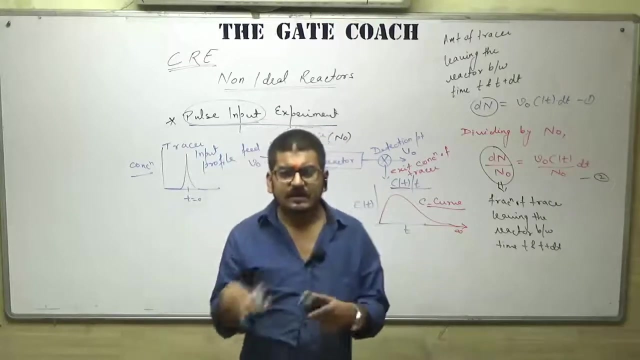 etc. so in all of the curves, when we analyze the distribution curve, there was one thing common: that we want to find out the mean value, median and mode, standard deviation and variance of the curves. ok, and all these things, all these parameters, we calculated or we calculate with the help of 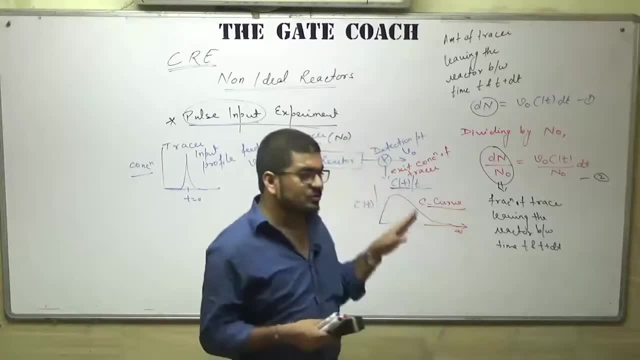 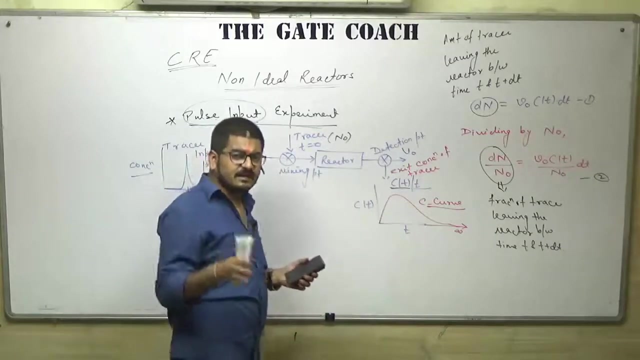 some distribution function there. in the same way, this residence time distribution, basically the application of probability distribution, all these things are based on probability distribution, but we will not talk about that because this is not the math class, this is the CRE class, so we will discuss that thing. 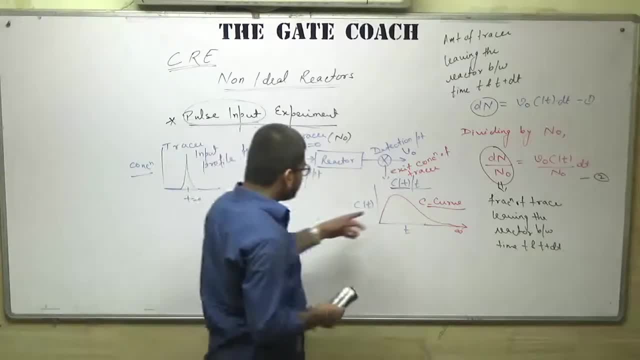 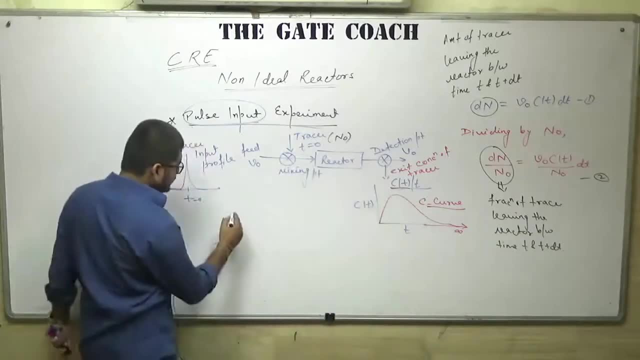 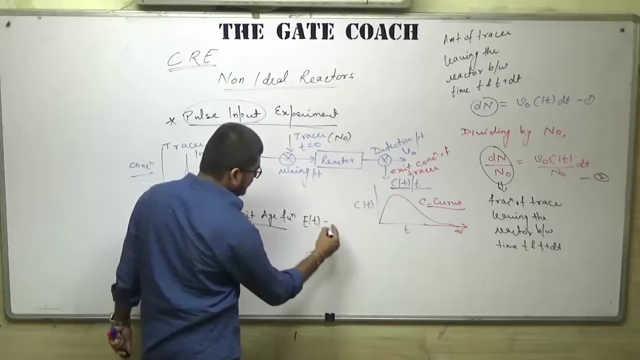 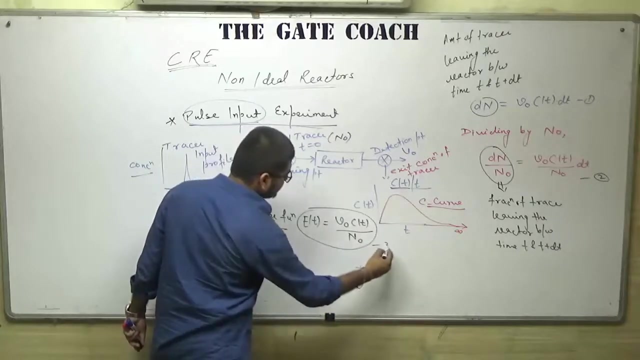 how to use that. so here as well, for this C curl, we will find out- we will define a distribution function known as exit h function. exit h function, which is like p0 into multiply by ct divided by n0. let's see equation 3: ok, and 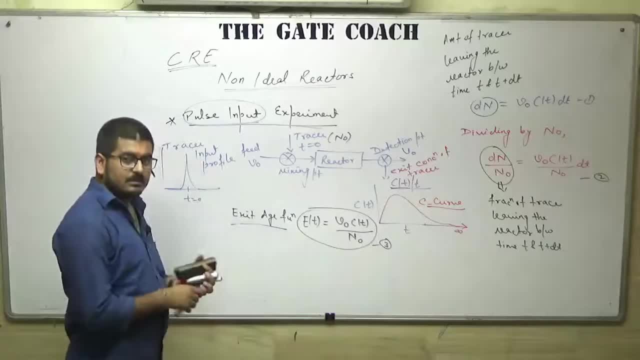 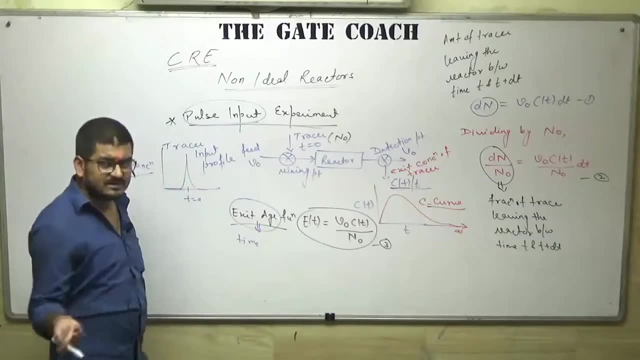 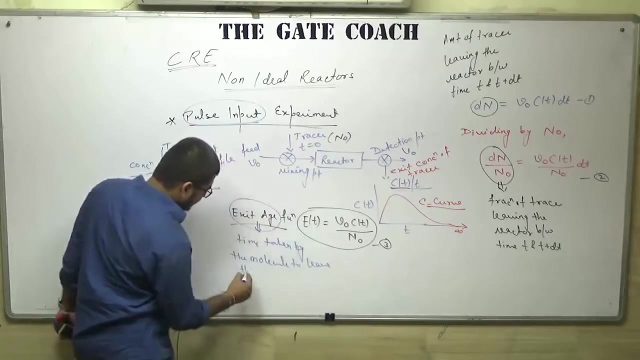 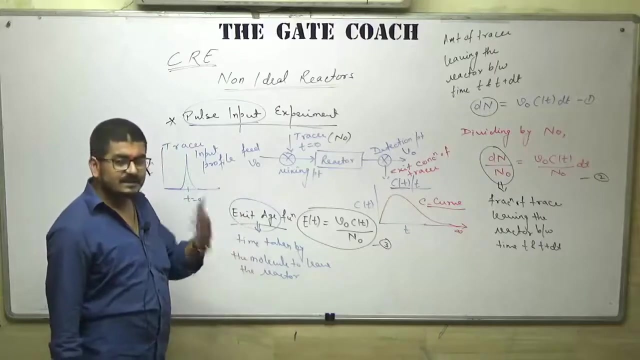 what is exit h? so exit h is can. it is just analogous to the residence time, but definition wise, we can say it is the time taken by the molecule to leave the reactor, time taken by the molecule to leave the reactor. so now see, it is just like the residence time. 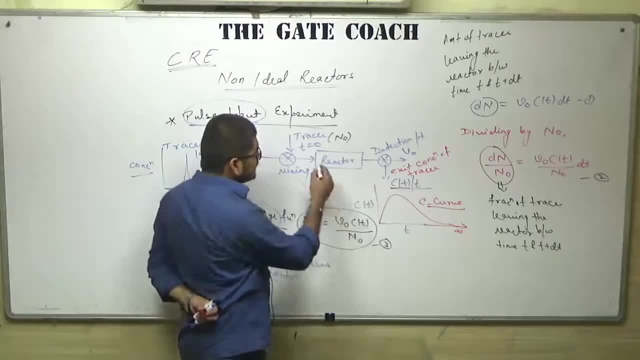 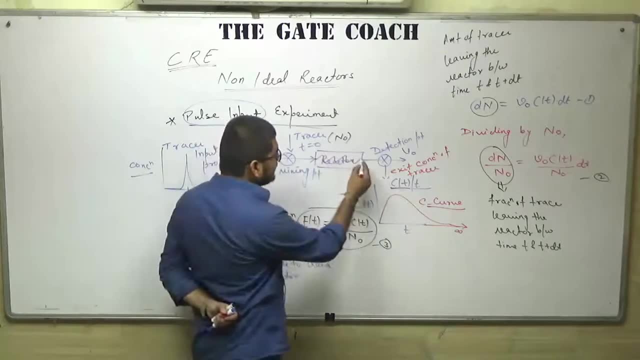 here residence time can be defined as the time spent by the molecule within the reactor. so when the molecule entered in the reactor, that is t equal to 0, and when it leaves the reactor, at time t. that duration we call residence time. but in the same way 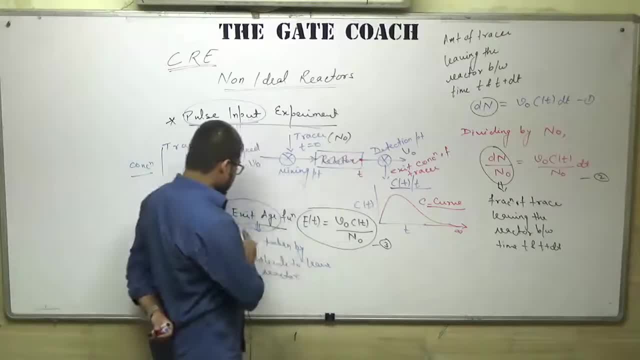 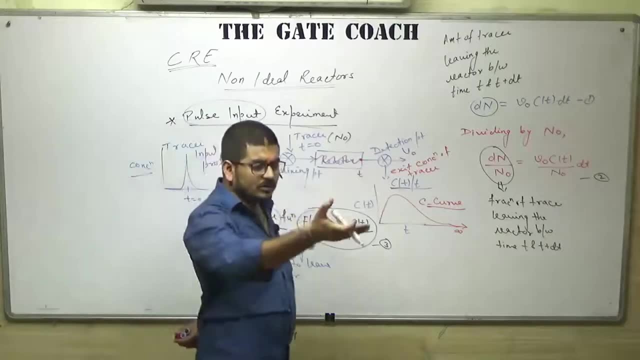 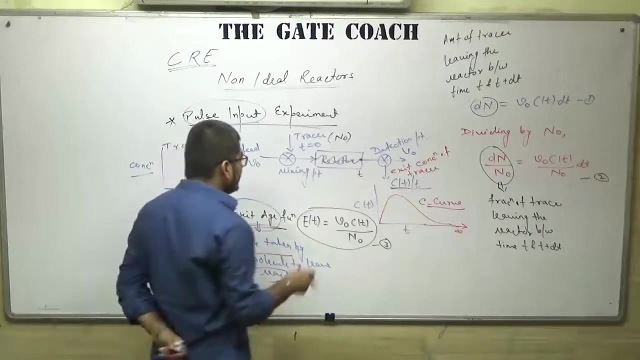 here in exit h function. exit h, which is the time taken by the molecule to leave the reactor, means we are waiting at the outlet to leave the. we are waiting at the outlet of reactor for the molecule to leave. ok, so what we are doing, as you can see. 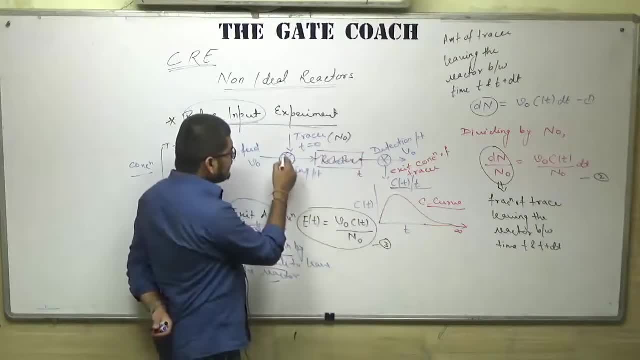 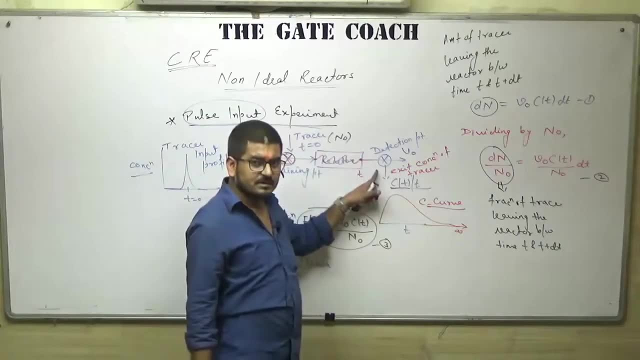 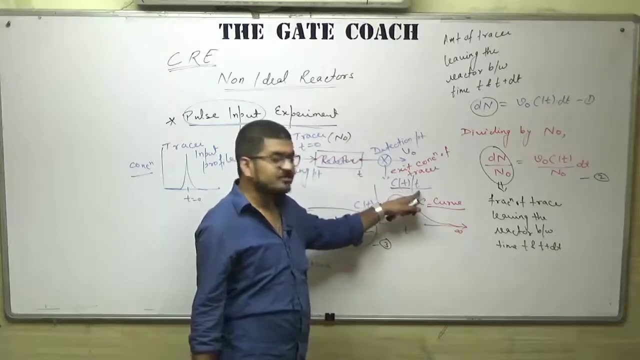 in this experiment, we are injecting the tracer at time t equal to 0 and it enters in this. ok, now we are waiting at outlet for the molecule to leave. and when the molecule will leave, we will calculate. we will measure their concentration with the help of titration chromatography. 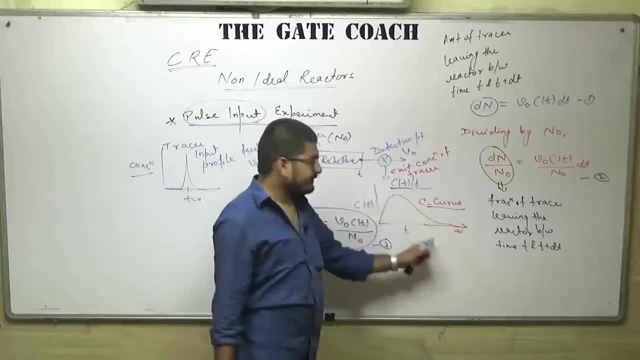 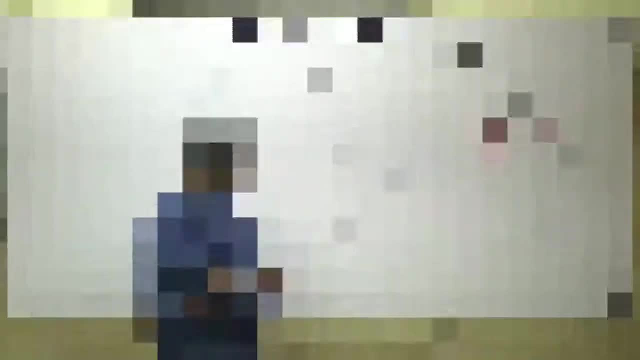 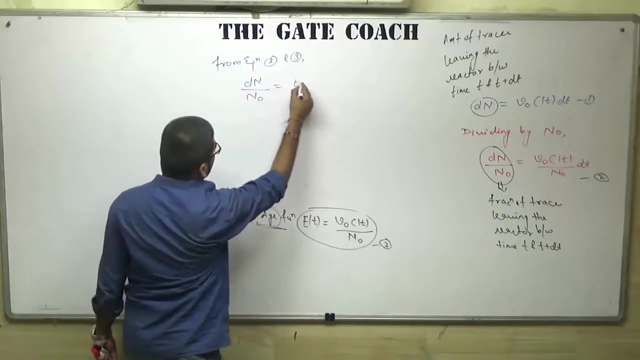 or n number of phase are there and we will draw the curve, and this is what we call exit h- time taken by the molecule to leave the reactor. ok, so from equation 2 and 3 it is clear that dn over n0 is equal to et into dt. 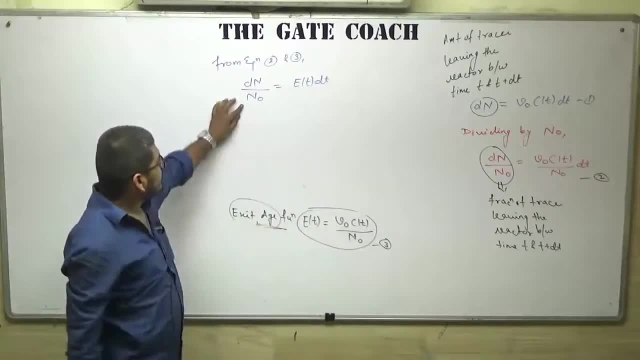 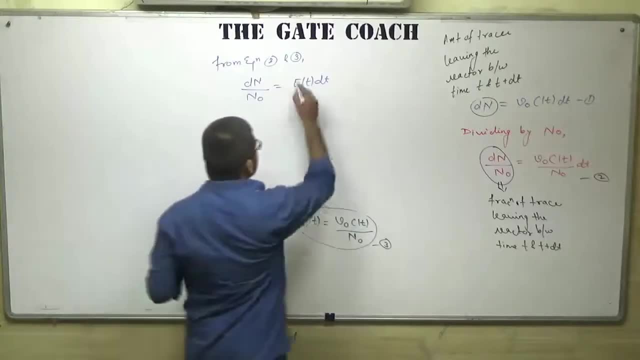 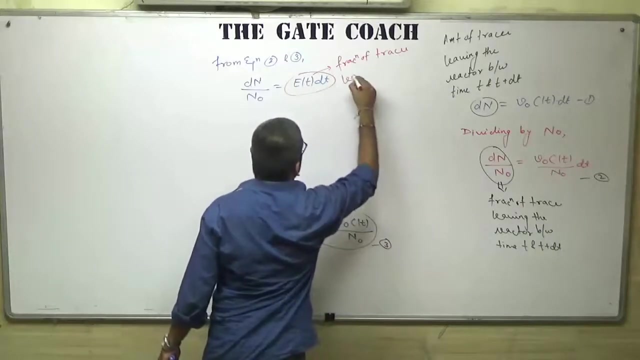 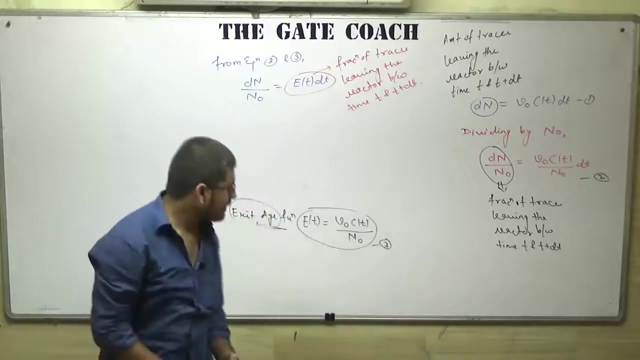 ok, and what is dn over n0? this is the fraction of tracer leaving the reactor between time t and t plus dt. in the same way, this et dt will also define as the fraction of tracer leaving the reactor between time t and t plus dt. ok, so 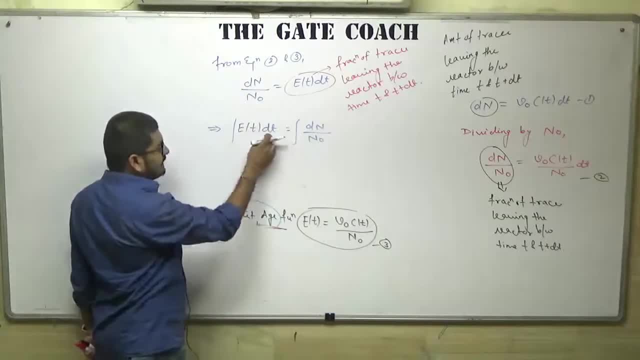 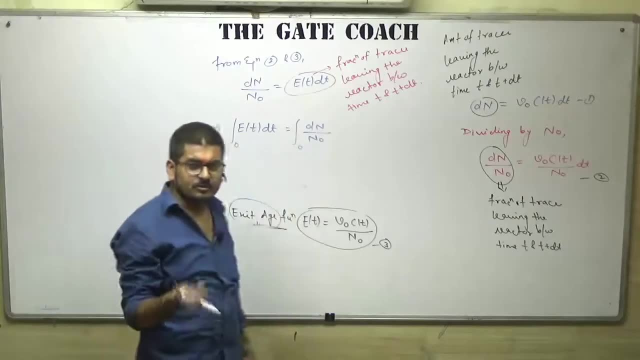 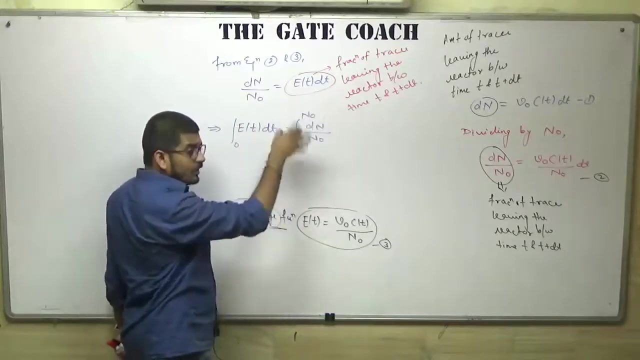 if you integrate this point, so at time t equal to 0, the molecules leaving the reactor will be 0, because at 0 we are injecting some molecules, so they will not leave, and the time required by the molecules, the time at which all molecules will leave. 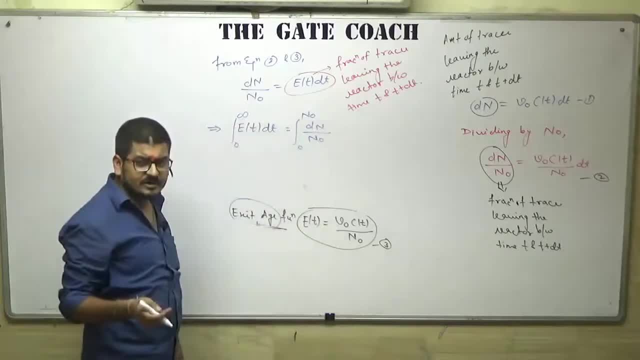 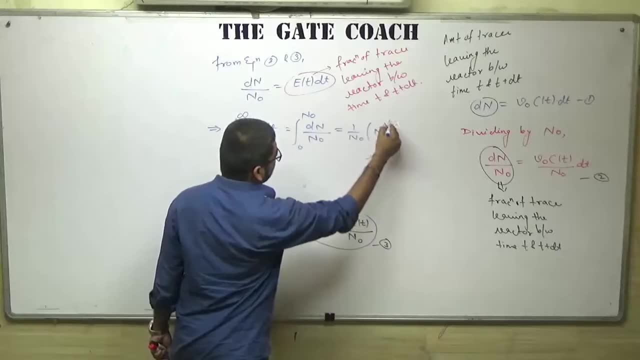 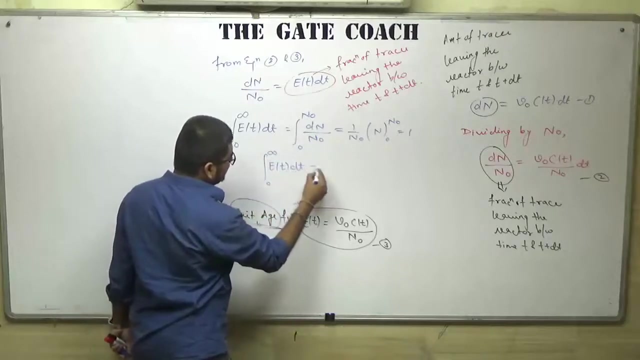 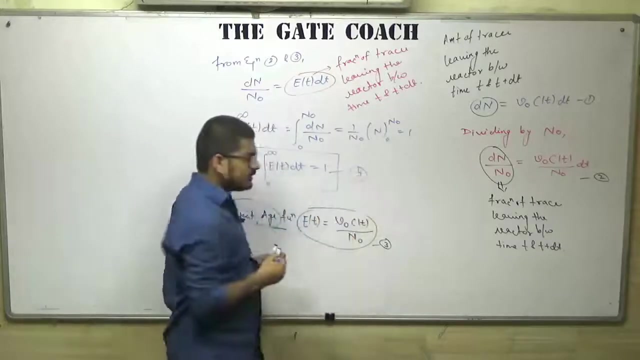 will be infinite because of the dead zone, and when you solve this it will be like: so you can write it as 0 to infinite, et dt is equal to 1. ok, and let's say this is equation 4. et dt was fraction of tracer leaving the reactor. 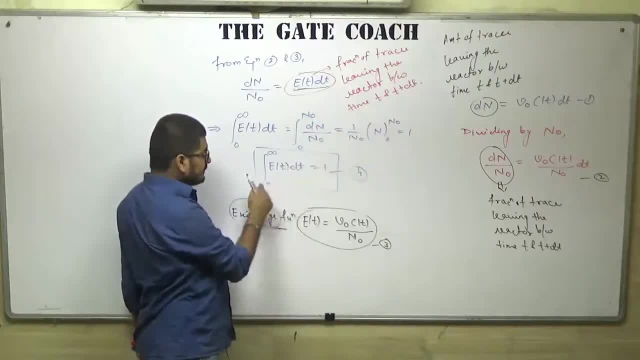 between time t and t plus dt, and when we integrate this from 0 to infinite means in total time interval, the fraction of tracer will leave the reactor will be 1, and it should be 1, obviously, in total time interval. all molecules will leave the reactor, so the fraction 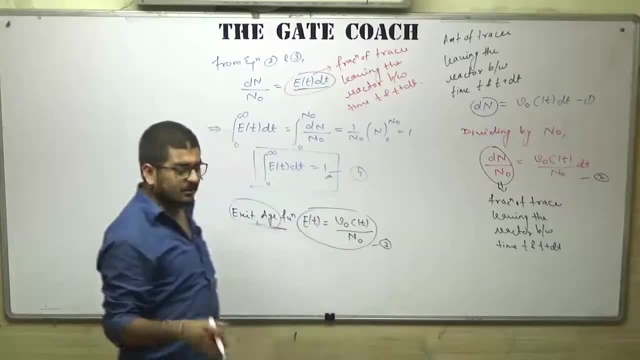 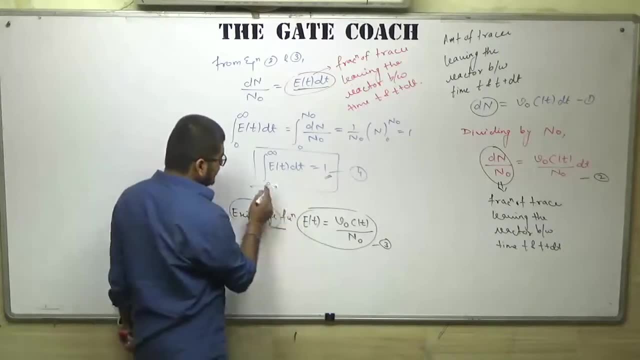 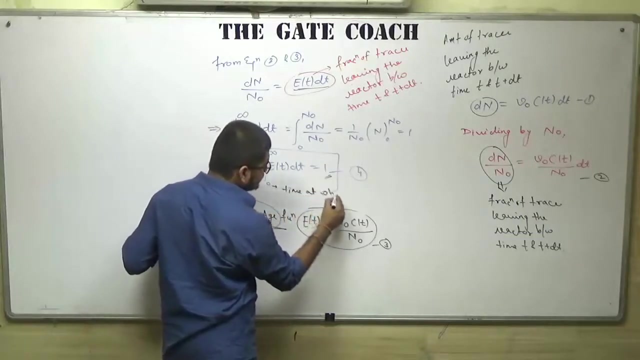 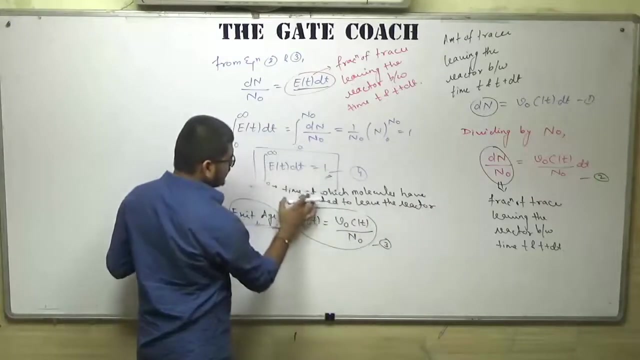 will be 1, so this is correct, ok, and here the 0 is the time at which molecules. here the meaning of this: 0, the initial limit is the time at which molecules have started to leave the reactor. actually, time at which means time after which- ok, and the infinite it means. 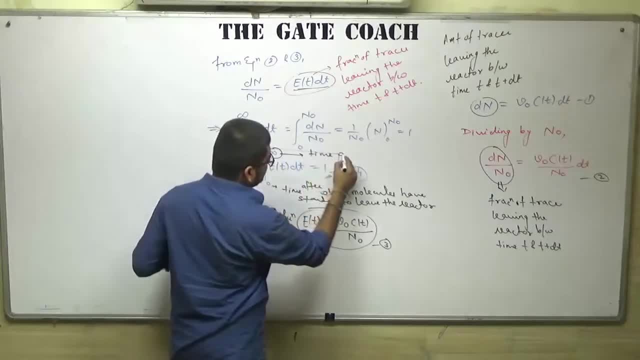 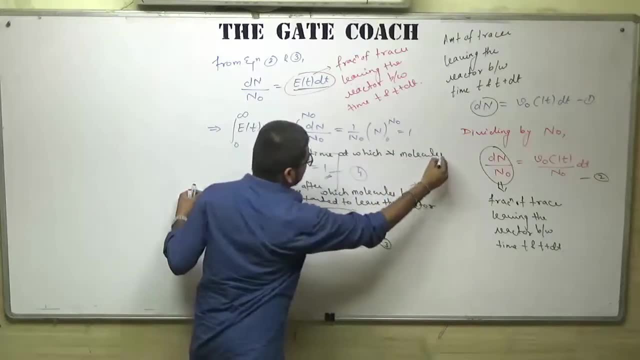 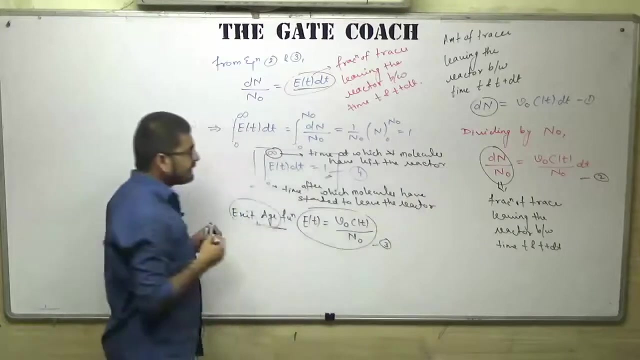 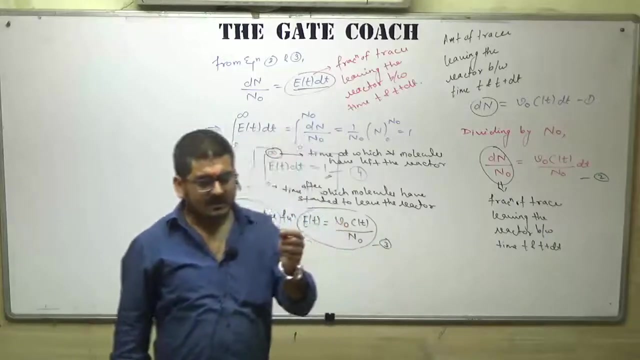 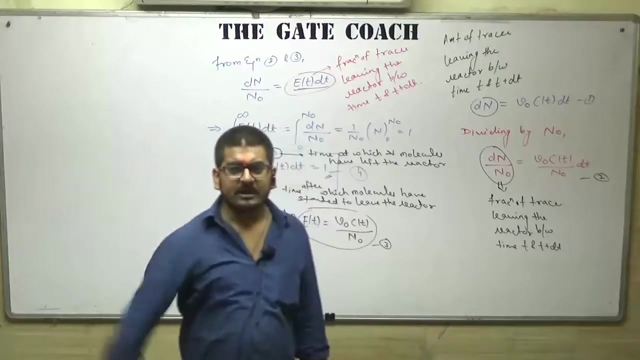 the time at which all molecules have left the reactor. ok, that is not the 0 and infinite can be also 3 and 25. ok, there is a reactor at t equal to 3 minutes, molecules have started to leave and all molecules will leave till t equal to 25. 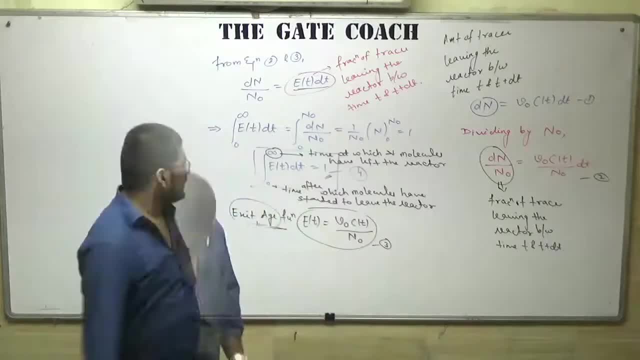 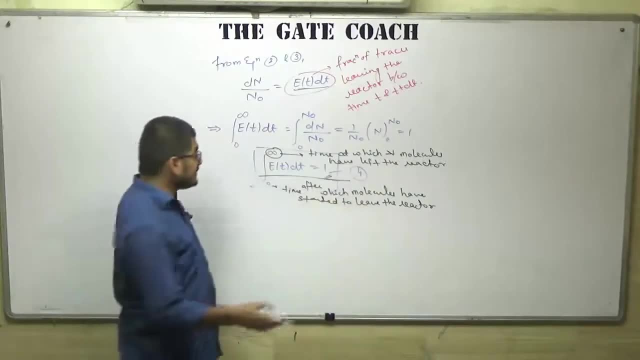 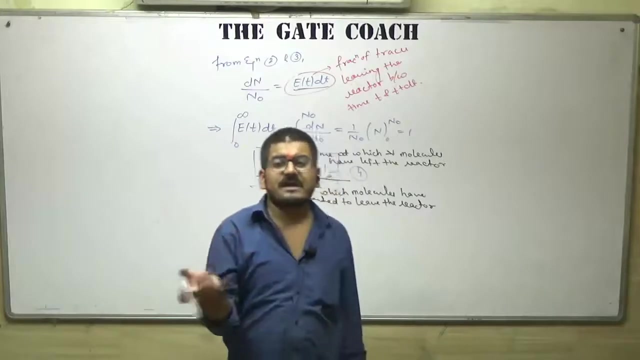 minutes. so the limits will be like that. ok, I think it is clear to all of you. ok, then now see this equation 4. this represents one more meaning, as all of us know the application of integration is. it also represents the area of some function means. in this curve it represents: 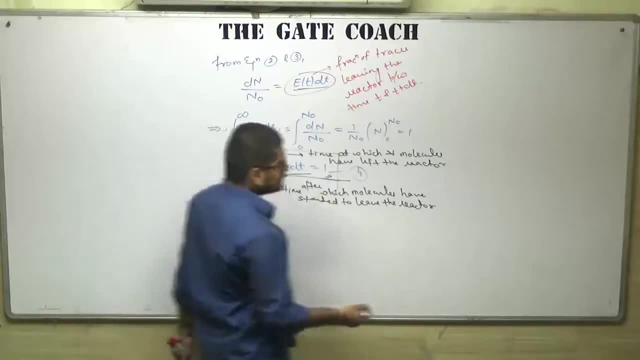 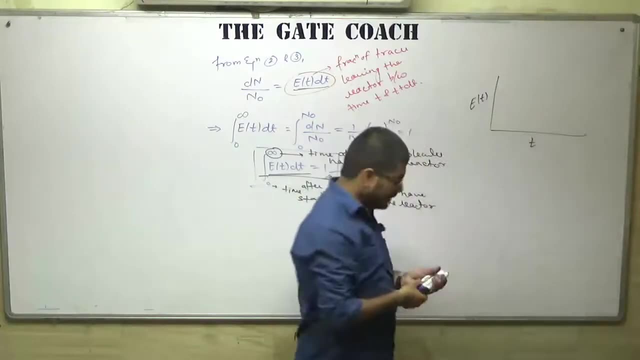 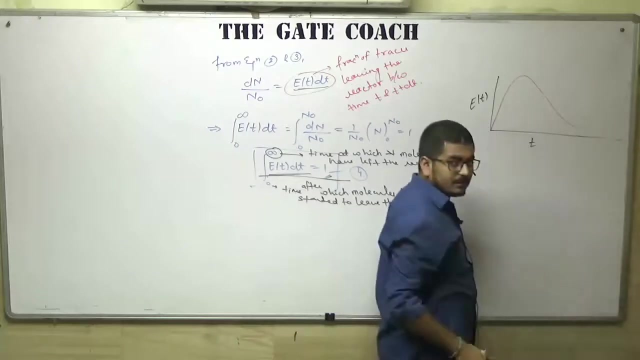 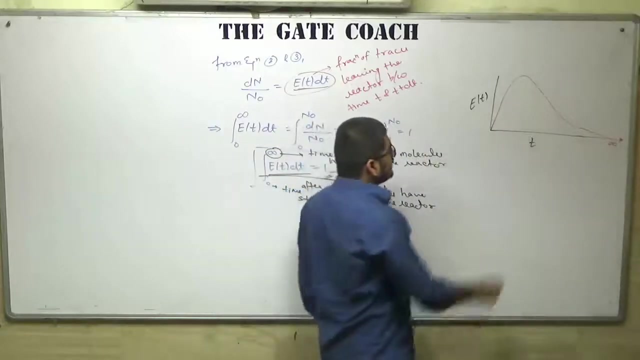 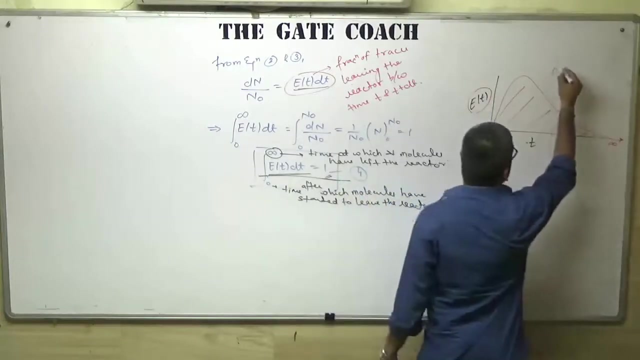 the area of this e versus time curve. so if we draw a curve between e versus time, so it will be like this, and this curve will leave at t equal to infinite, will touch the x axis. ok, in the curve drawn between e, exited function versus time is known as: 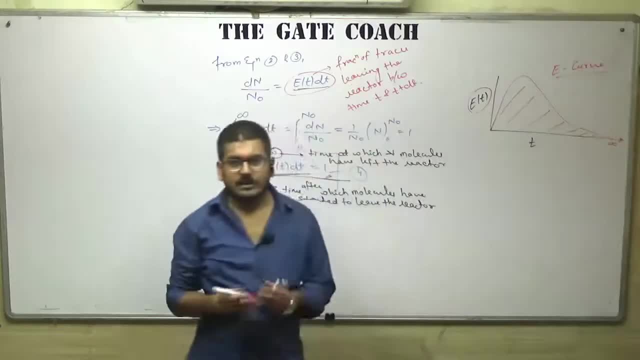 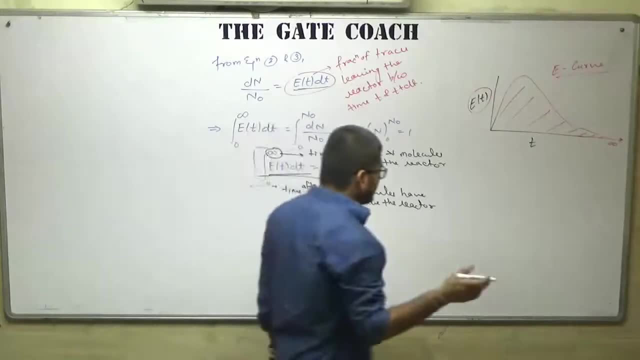 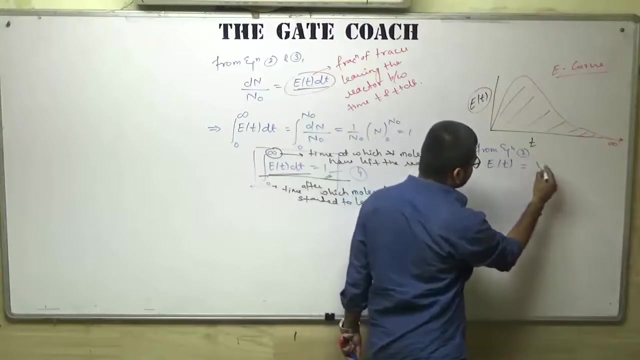 e curve. ok. now I think you will think that why the shape of this curve is like this. so if I say that, remember equation 2 from equation 2 e, t was like v0 over n0 multiply by ct. ok. and the c curve was like: 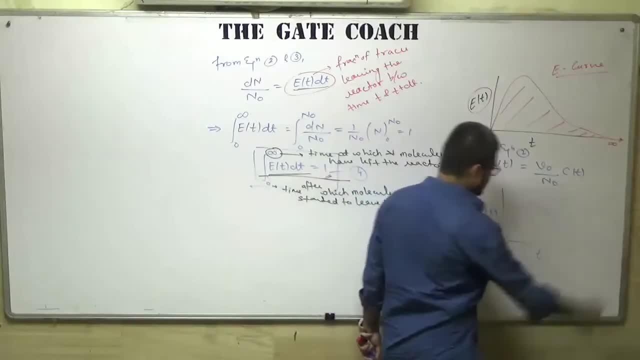 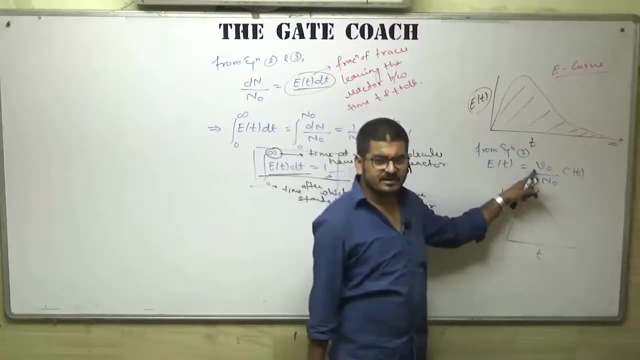 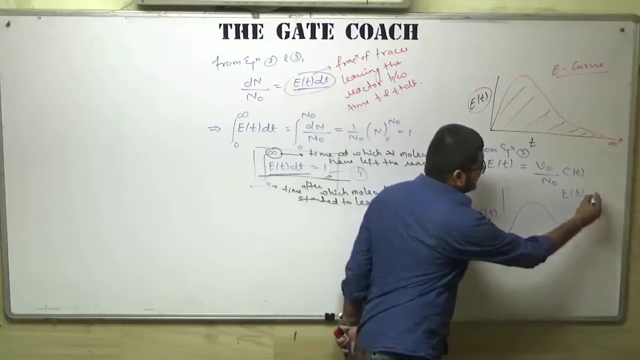 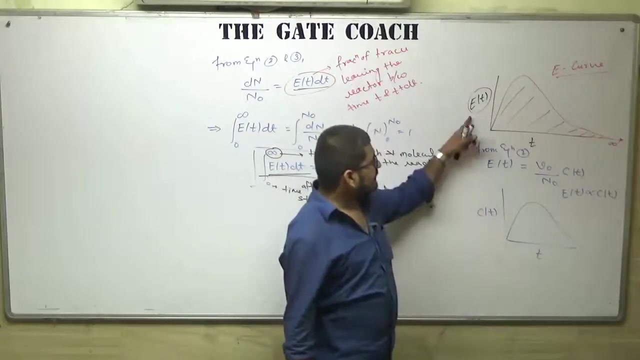 this so you can see. v0 is constant because the steady state reactor is there. n0 is the total amount of tracer molecules, which is already constant. so we can see that e t is directly proportional to ct. ok, and that is the reason. the nature of e curve will be same as. 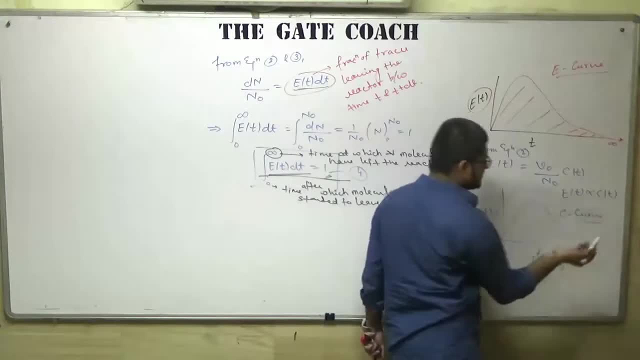 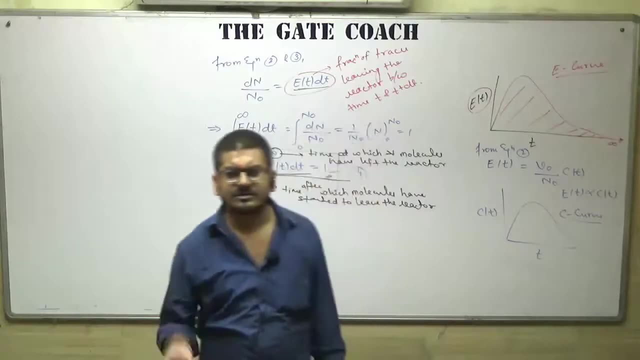 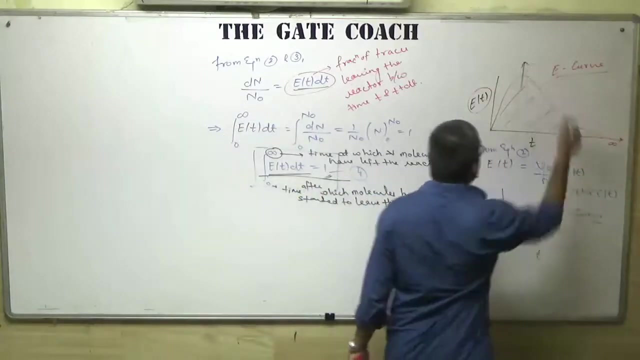 that of first c curve. if c curve is linear, then e curve will be linear. if c curve is parabolic, e curve will be parabolic. if c curve is triangular, e curve will also be triangular. ok, and what is the area of e curve? so you can see from this curve. 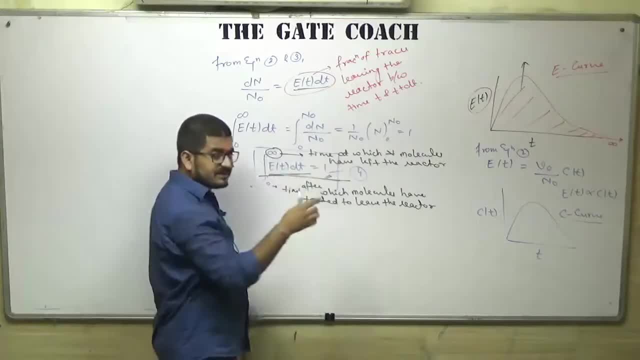 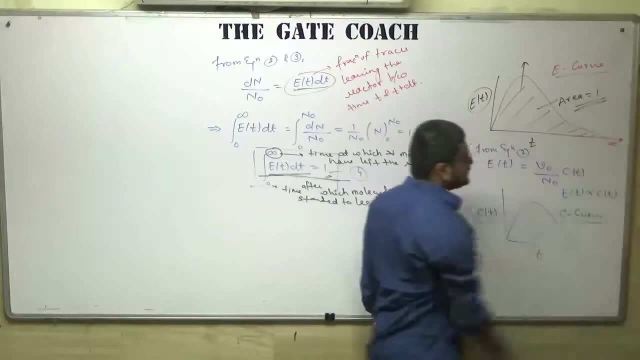 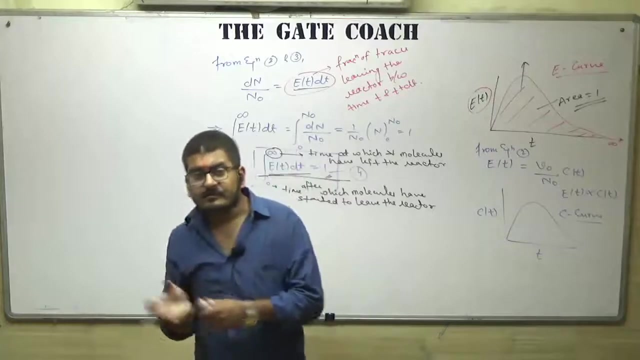 this equation 4 that from limits 0 to infinite means, in total time interval, the area of this curve will always be 1. ok, so remember this guys. this is a very key point in this study: that area of e curve will always be 1 for the total time interval. 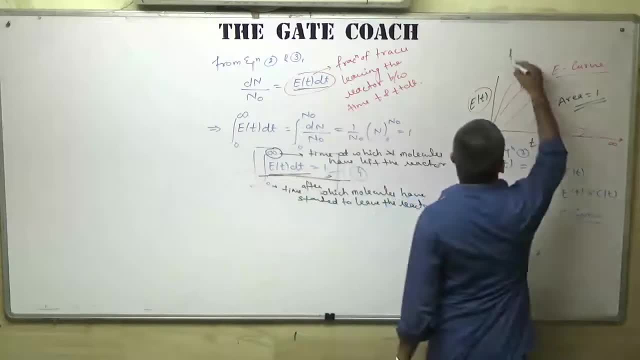 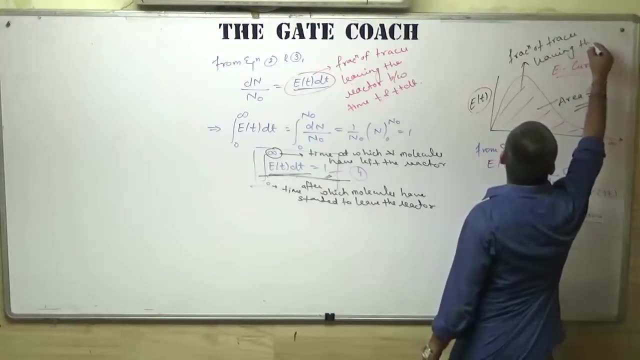 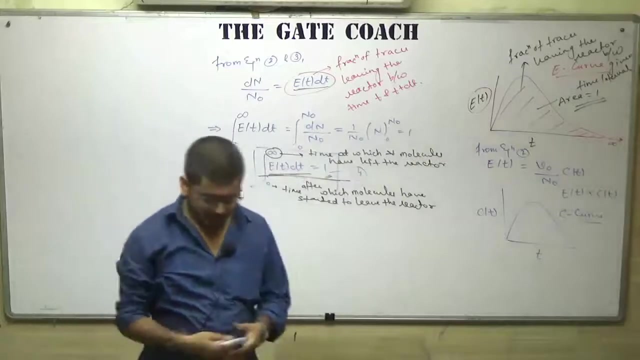 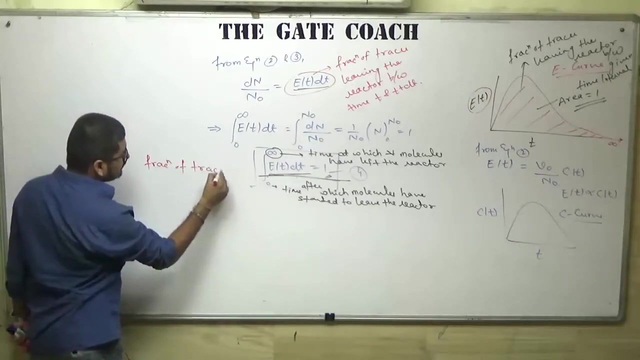 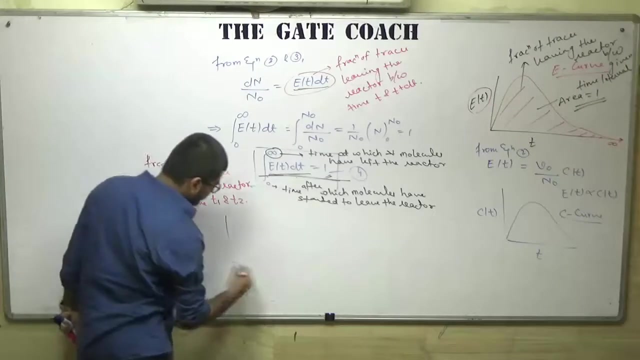 ok, and the area of e curve represents the fraction of molecules, fraction of tracer leaving the reactor between given time interval. ok, so if someone ask you to calculate the fraction of tracer leaving the reactor between time t1 and t2, so it would be like something like this: 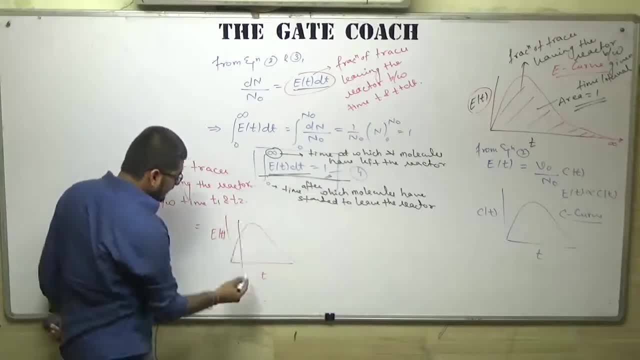 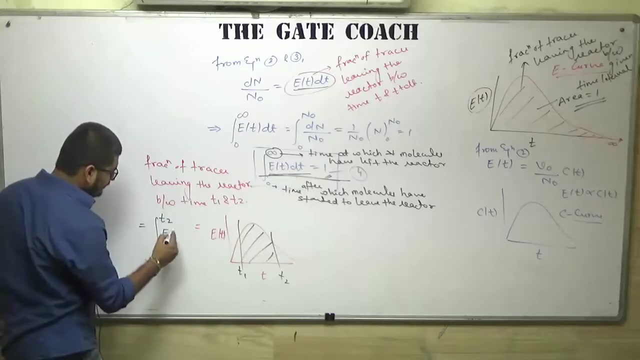 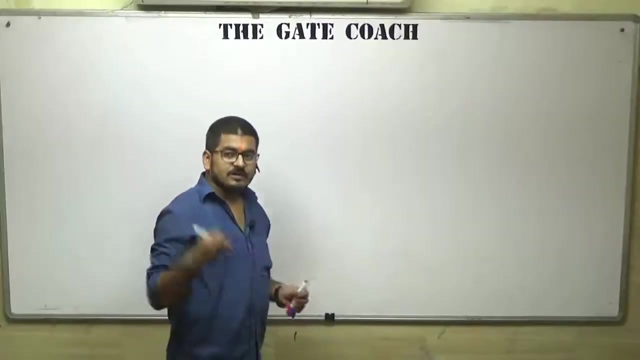 so just calculate the area of curve between time t1 and t2. or you can write it as mathematically: integration of t1 to, from t1 to t2 of et, dt. ok, now there is one more thing, that what will be the mean value of the curve? 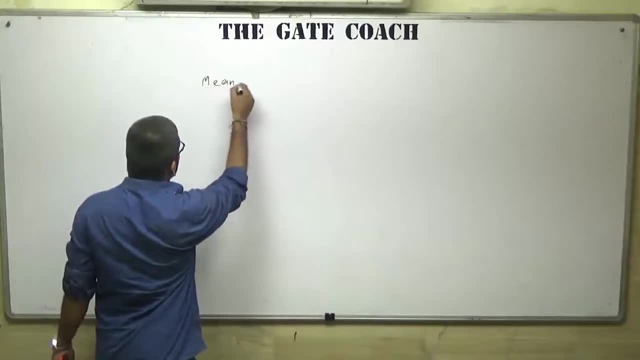 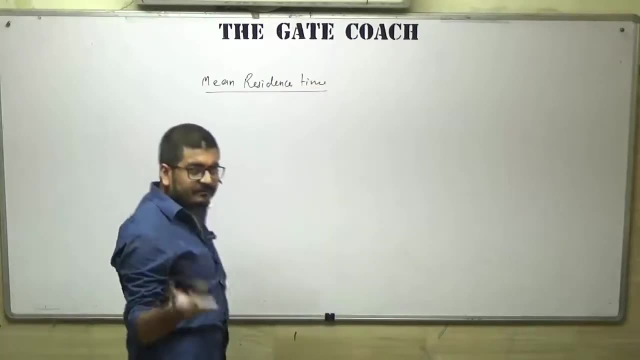 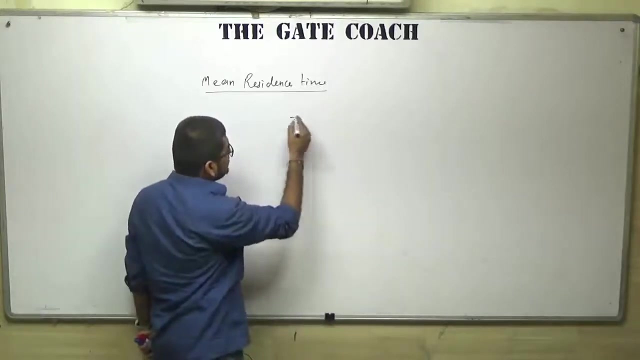 ok, or we can say the mean residence time. we have different molecules with different residence time. so what will be the mean residence time of total reactor? so we can denote it by that value, mean residence time, by t bar, and we know that mathematically the average of any term. 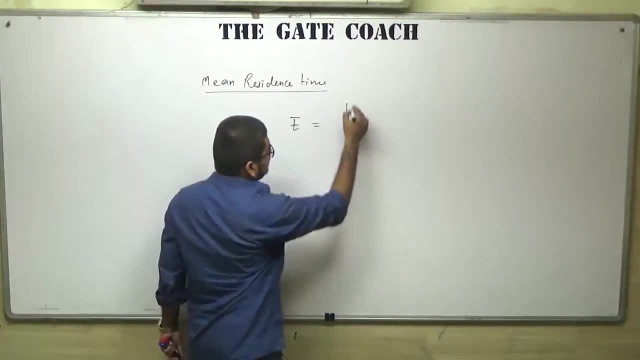 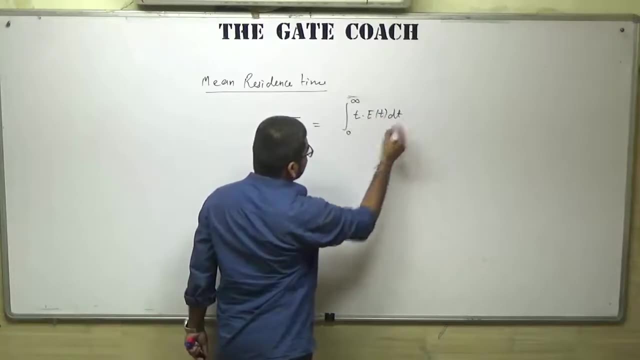 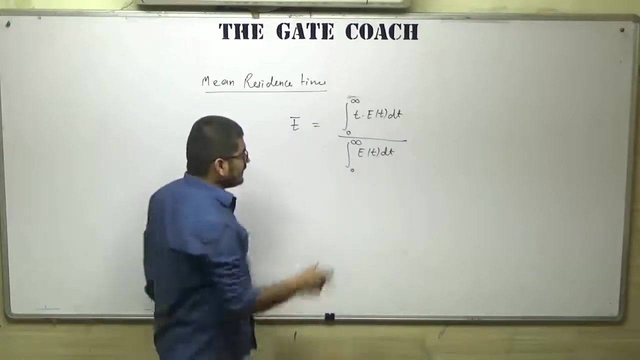 will be based on integration, and here the distribution function is et. so based on that we can define the mean residence time. ok, but the value of this curve, this function, et dt from 0 to infinite will be 1, so t bar will come out to be: 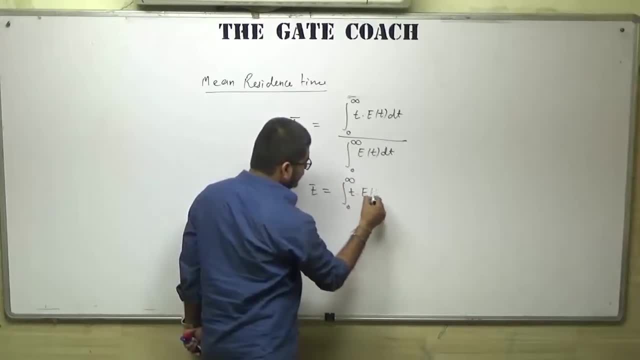 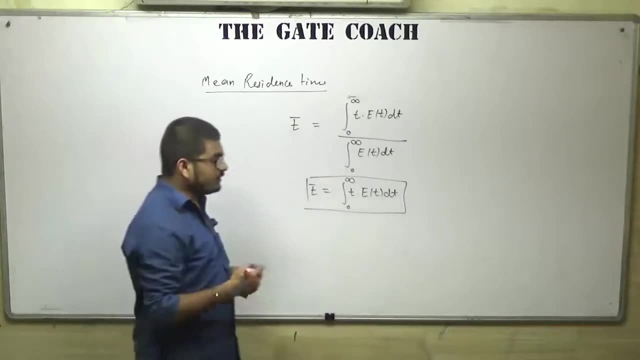 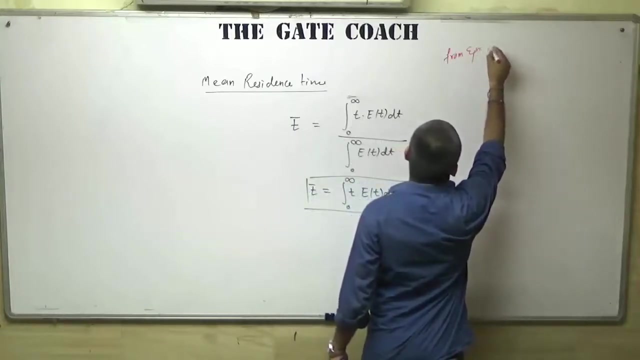 0 to infinite, of t into et, dt. ok, and now we know that in industry we are dealing with mixture, so we define normally concentration terms. we don't deal with moles for the mixtures. ok, so the exit from equation 1. you know that we were having 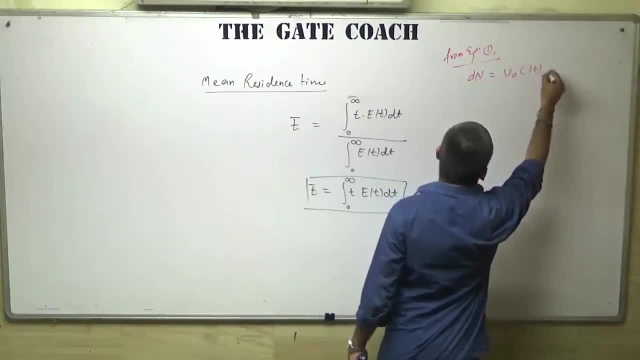 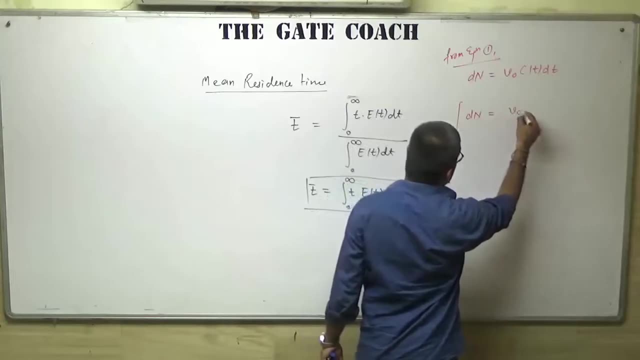 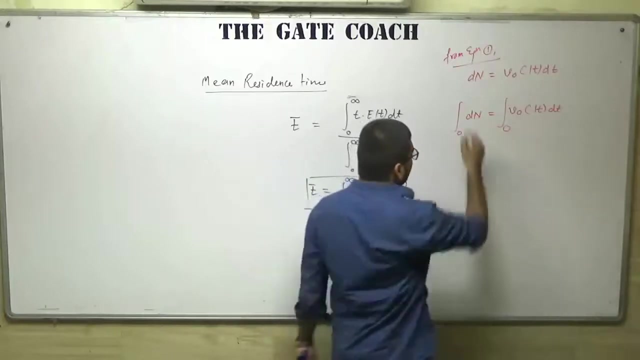 dn is equal to v0 ct into dt. so if you integrate this function you will get: dn is equal to v0 ct into dt. so at time t equal to 0 molecules leaving the reactor will be 0, and time required by the molecules- all molecules- to leave the reactor will be. 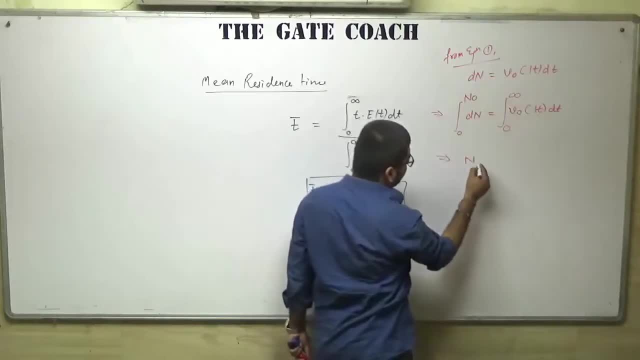 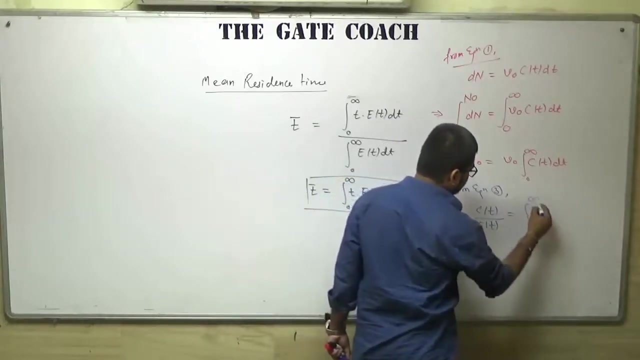 infinite. ok, so it will be like: n0 is equal to v0, integration from 0 to infinite. ct into dt. and now from equation 3, if you know that n0 over v0 can be written as: ct over et is equal to 0 to infinite integration of. 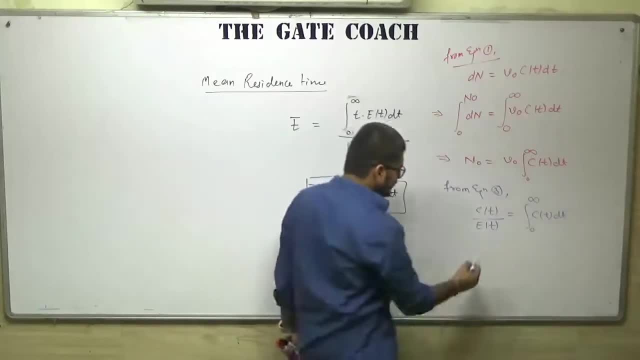 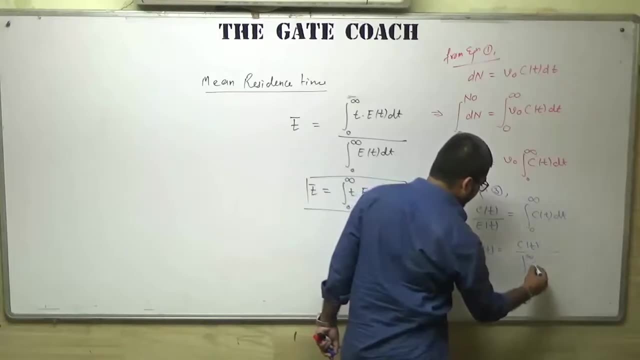 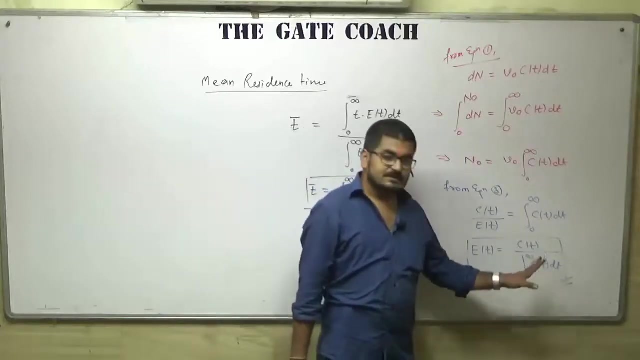 ct, dt. ok. so et will come out to be like ct over integration, from 0 to infinite of ct, dt. ok, write any question: 5,6 or whatever, it is ok. so now see, et is equal to ct over this. and what is this part denominator, integration of. 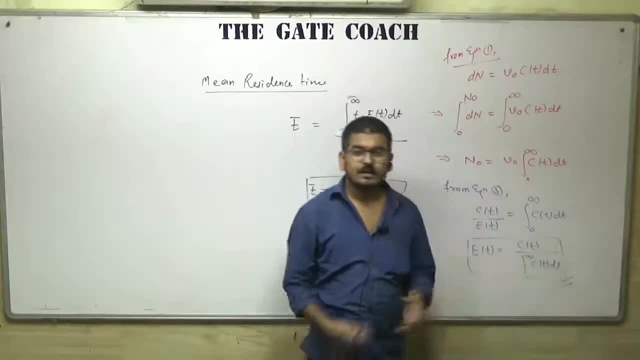 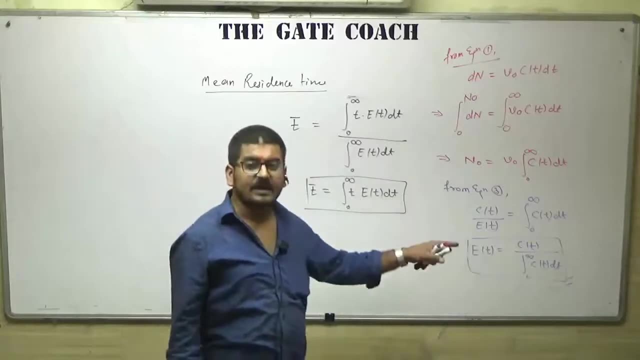 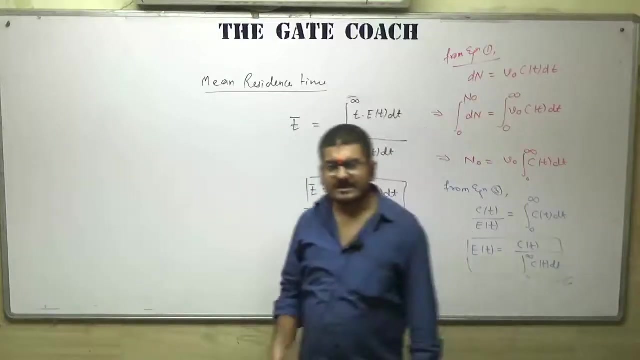 ct, dt from 0 to infinite. and what is ct? ct is the concentration of tracer at exit of the reactor, means, it is a result, and this is basically the area of c curve. now tell me one thing: all of you must have cleared your 12th and 10th examination. 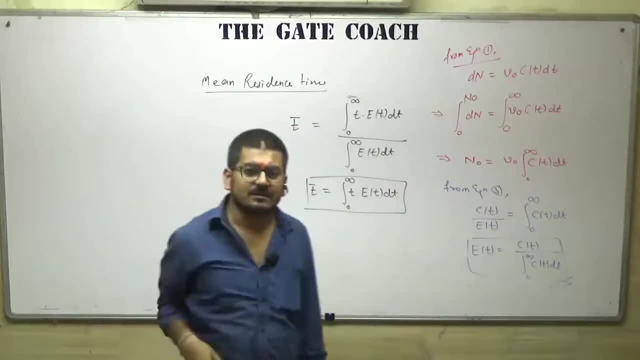 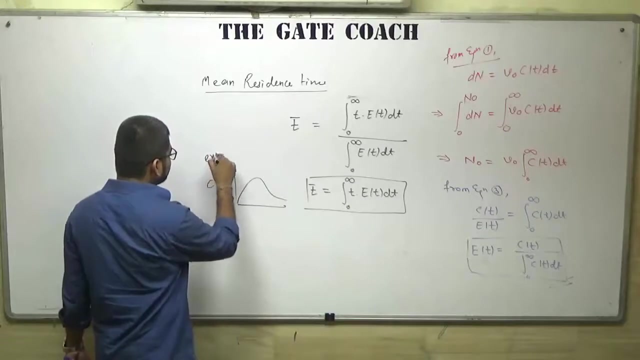 so can you change your 10th result, the value of 12th result? no, obviously, because those are results and those are constants. so, in the same way, in c curve, which is the curve between exit concentration of tracer versus residence time, which is our result. so this area, 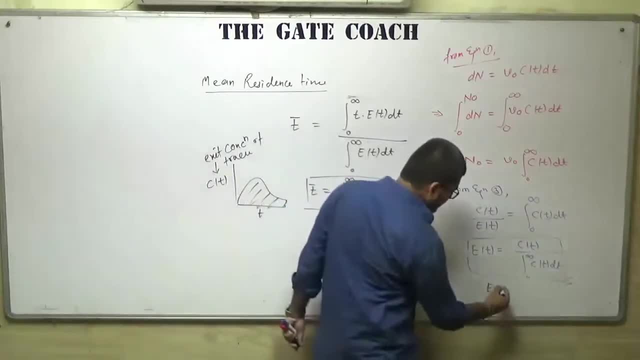 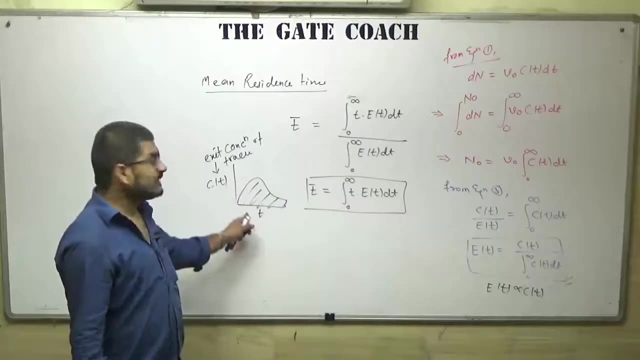 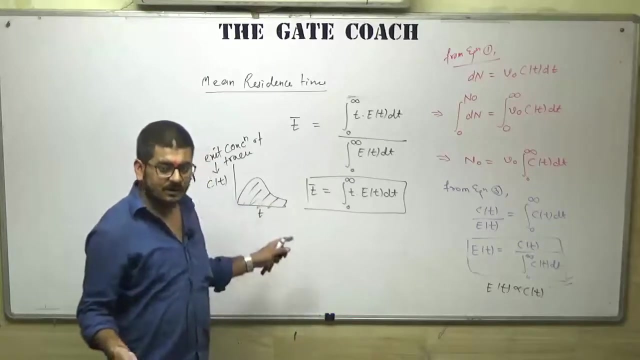 will be constant. so, ultimately, et is proportional to ct. because this is constant, because that is the area of c curve and c curve is the result, outcome of the process. so the values will not change after coming out. ok, so now, when you put that value in this equation? 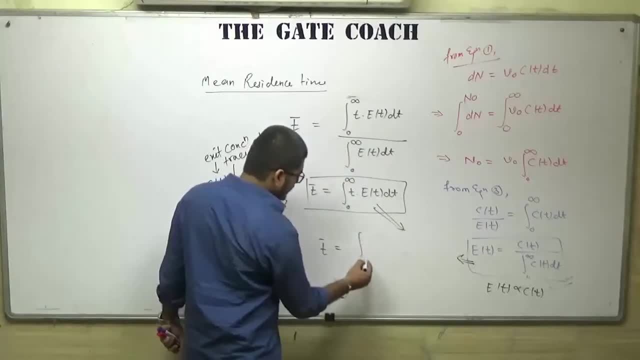 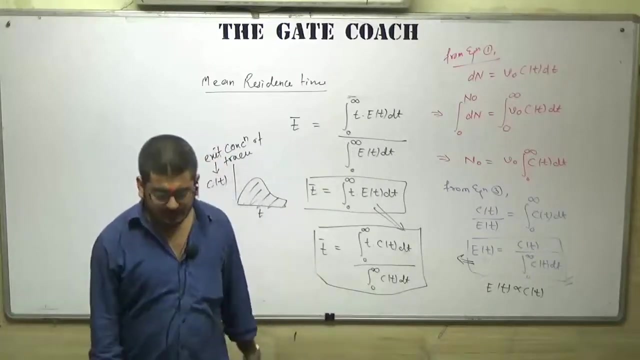 you will get. t bar is equal to integration from 0 to infinite of t into ct. dt divided by integration from 0 to infinite of ct into dt. so this is one way to find out the mean residence time. so this is something about pulse input experiment and all. 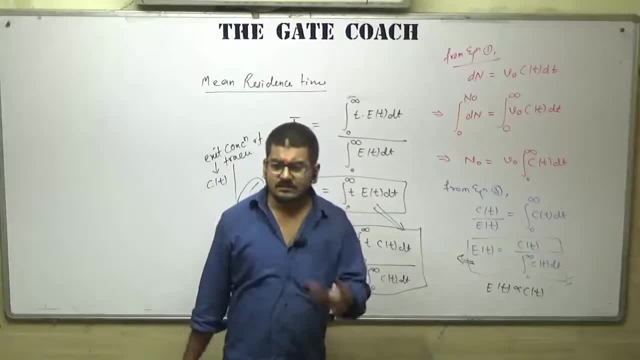 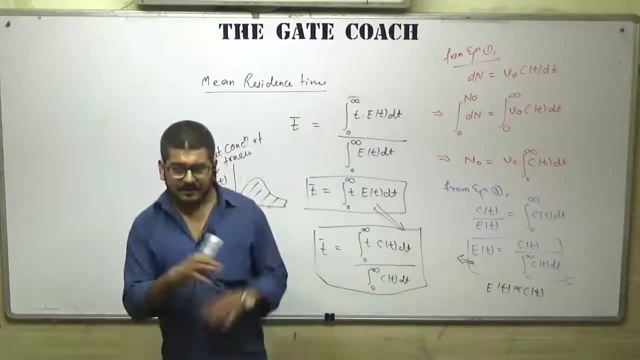 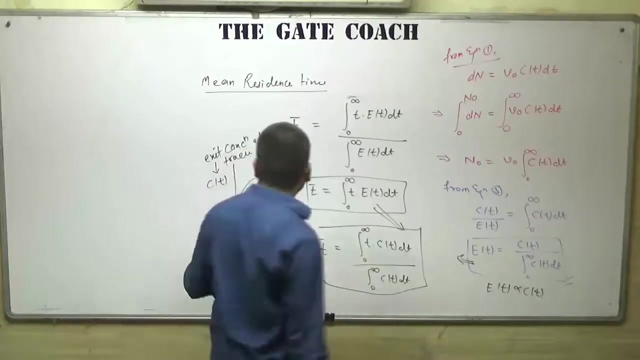 there are so many points to discuss that we will discuss in class, or if you have any doubt, then you can ask that in your comment section. now I am just wrapping all this by solving our numerical from the gate examination, which came in the gate exam from 2005 or 2006. 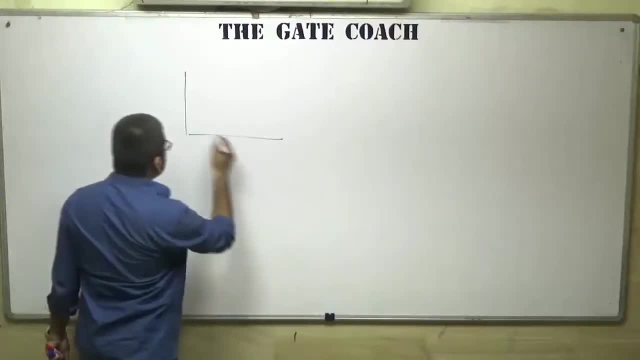 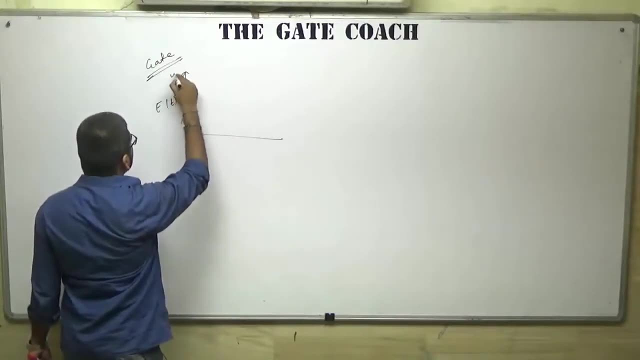 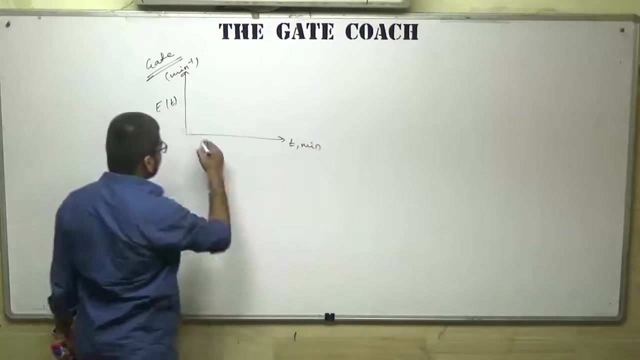 ok, so there was a question in gate exam that we have given our e curve. the units of function is minute inverse versus time, that is, in minutes. ok, the curve is something like this: ok, this is 3, 8, 15, 0 and this value was emax. 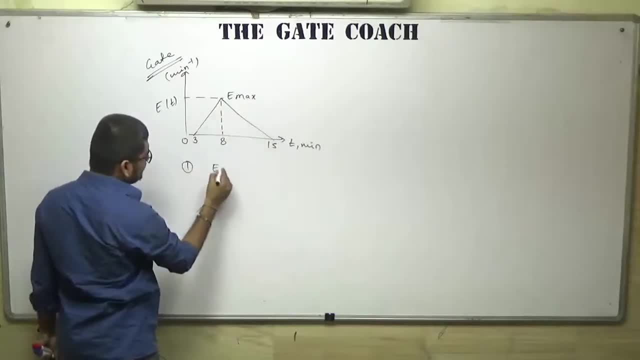 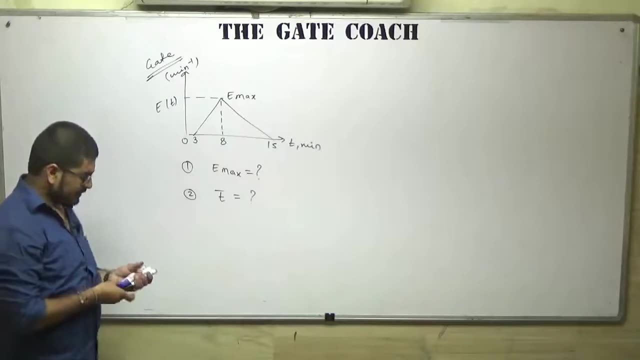 so I asked you first what is the value of emax and second, what is the value of mean residence time. so this question was there for 4 marks, 2 plus 2 sorry. so it is a very simple question. for a pulse input experiment, rtd curve was given. 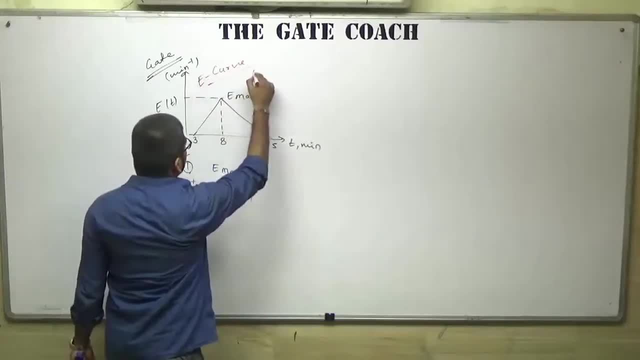 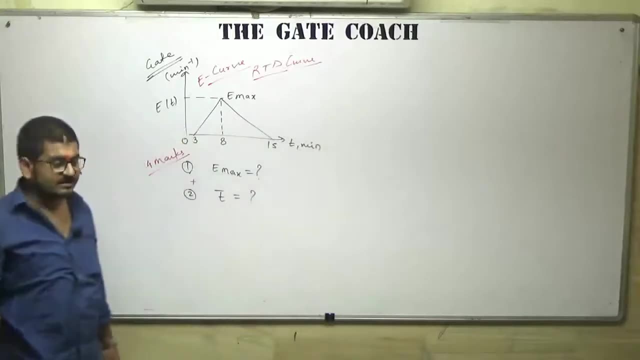 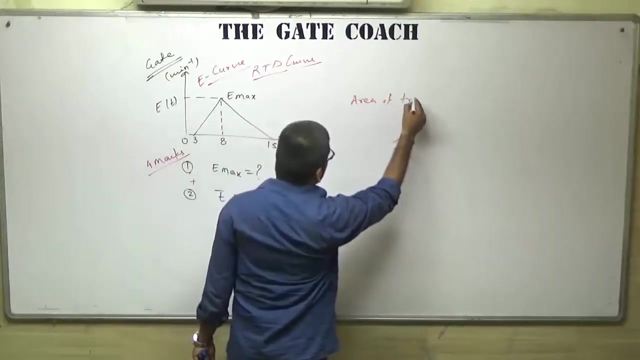 this e curve is basically known as rtd curve of the reactor. ok, remember this. so now you have to calculate emax. we don't know how to calculate that, but we can see it is a triangle and we know that area of a triangle can be written. 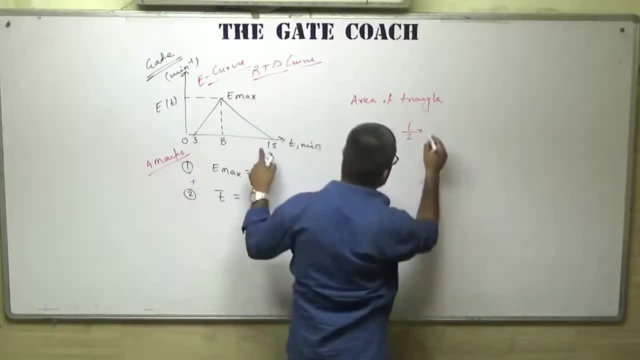 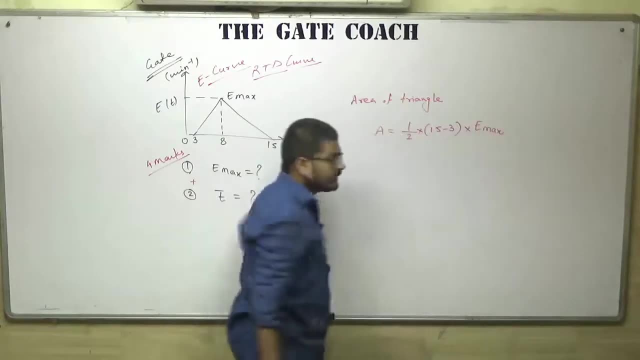 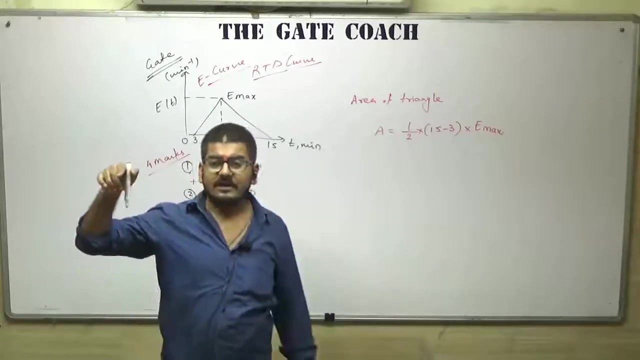 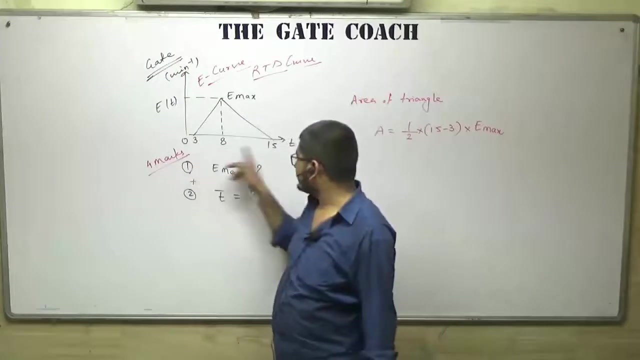 calculated by half into base, into height. ok, and because from the definition of e curve we just calculated that the area of e curve in the total interval will be 1, always. so here, in the total interval from 3 to 15, the area of e curve will be: 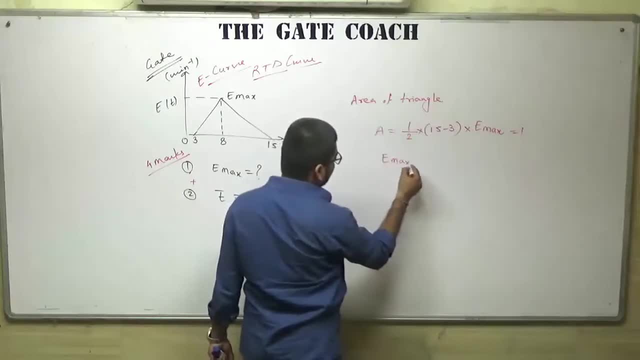 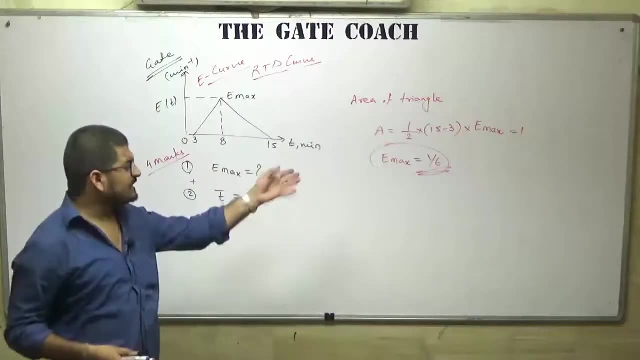 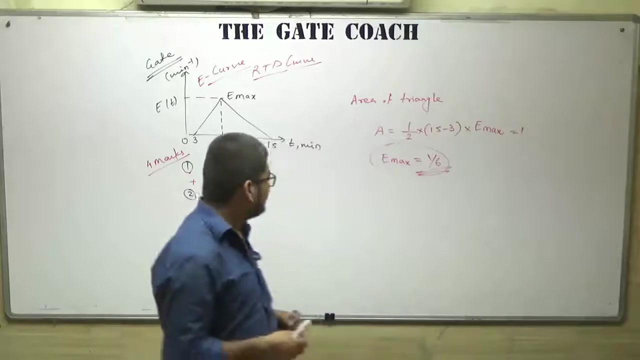 1. so the value of emax will be 1 by 6. very simple, this question was there for 2 marks. ok, you can imagine which kind of question came in exam. ok, very basic, conceptual question. next is t bar mean residence time. so we know that. 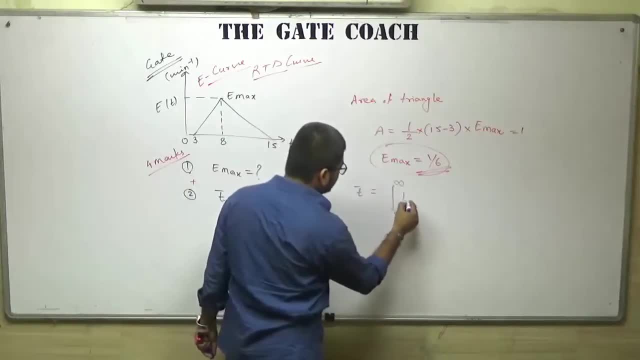 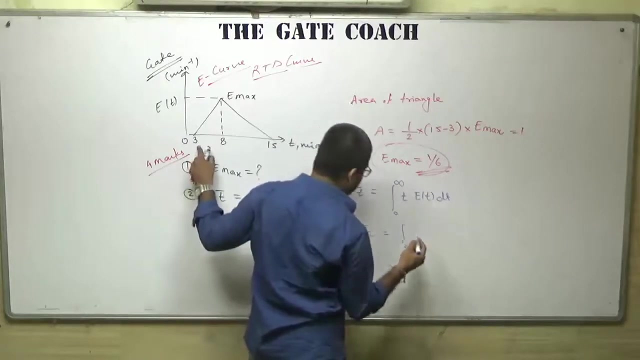 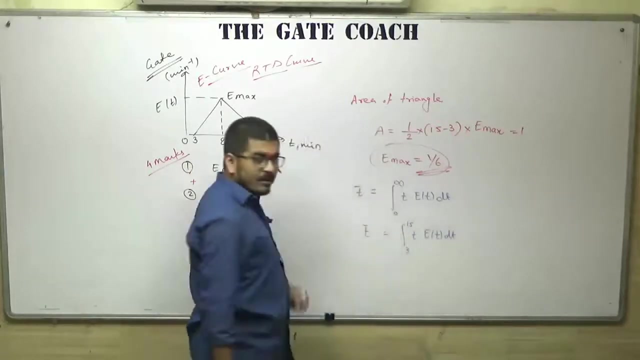 t bar can be calculated by the equation like this: ok, so for this curve the equation will become: the time after which molecules started to leave the reactor is 3, the time till which molecule left the reactor 15 t into e t dt. ok, but now we can see. 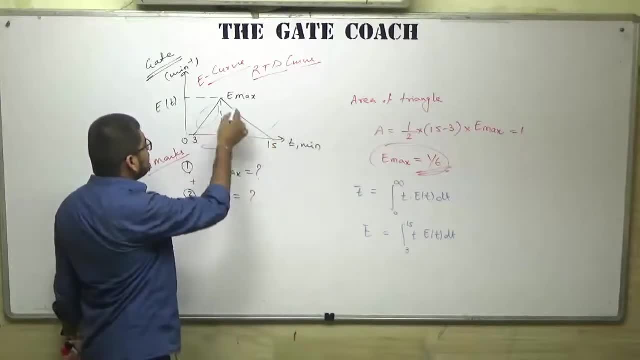 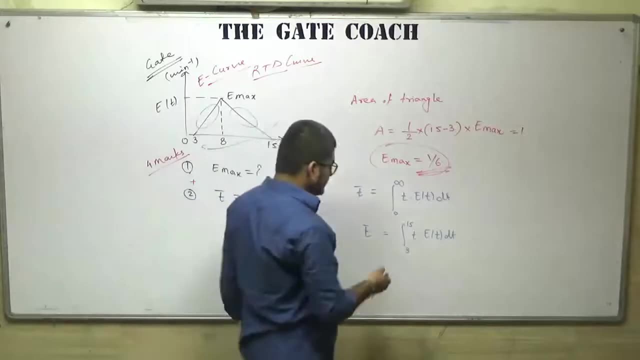 in this function, in this curve there are 2 slopes. curve is changing. ok, slopes are changing between the time intervals. so this t bar can be written as integration from 3 to 8 of t into e1 t, dt plus integration from 8 to 15. 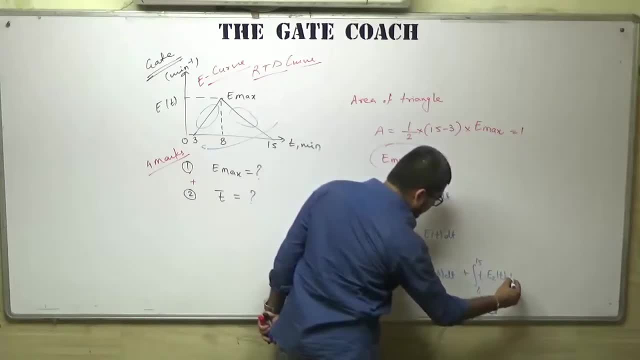 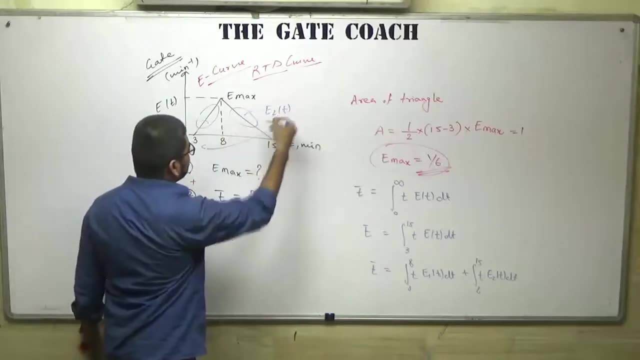 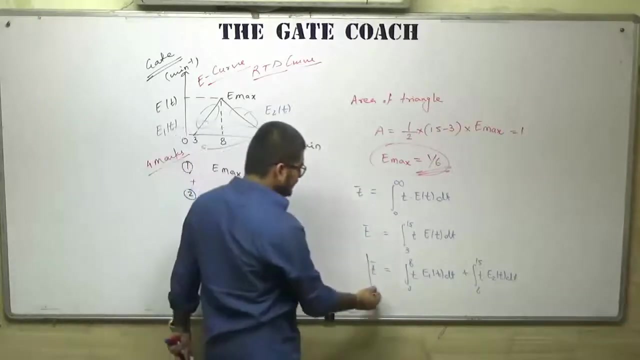 of t into e2, t, dt. lets say, this part is e1 and this part is e2 t. ok, put the values of e1 and e2 as a function of time in these in this equation and you will get your answer. ok, now how to find out. 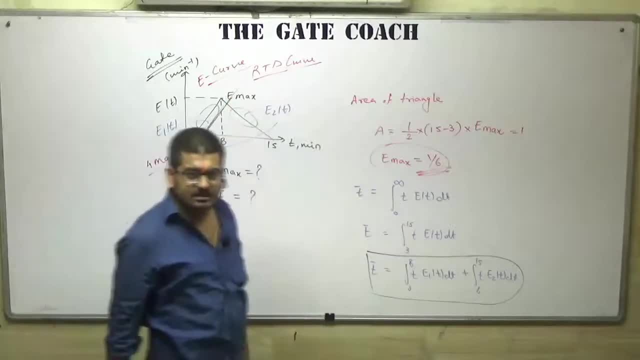 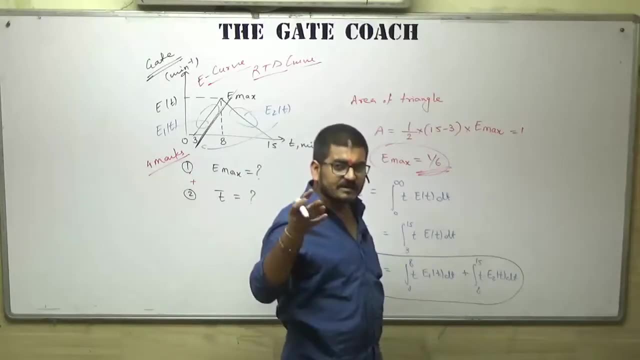 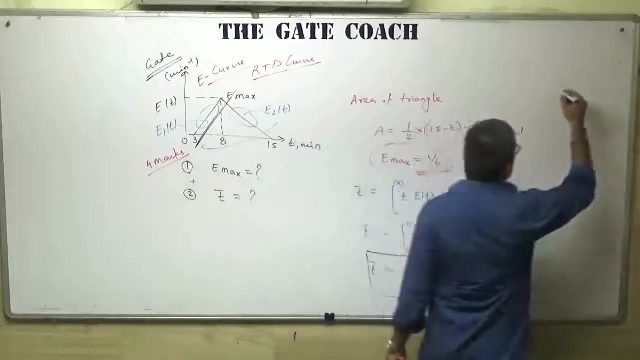 see, this is what a straight line equation and we straight line curve and we know that the equation used to represent the curve straight line curve connecting between 2 points will be like: y minus y1 is equal to y2 minus y1 over x2 minus x1. multiply by. 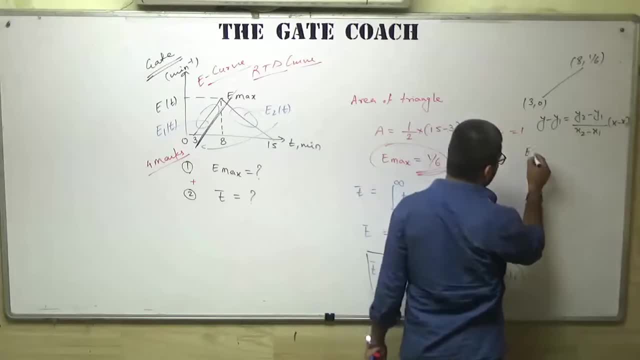 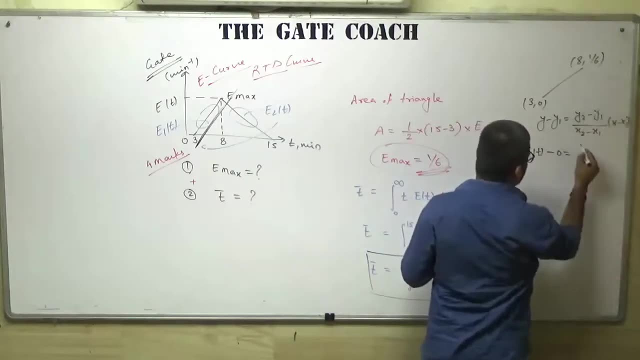 x minus x1. ok, so for this case it will be like: on y axis we have e, e1, t minus y1, that is 0. y2 minus y1, that is 1 by 6 minus 0. x2 minus x1, that is. 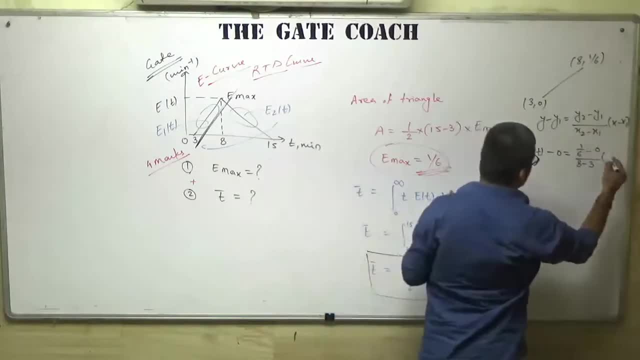 8 minus 3. on x axis we have t, so it will be t minus x1, that is 3, so here you will get e1. t is equal to 1 over 30 t minus 3, and which is valid for time between 3 to 8. 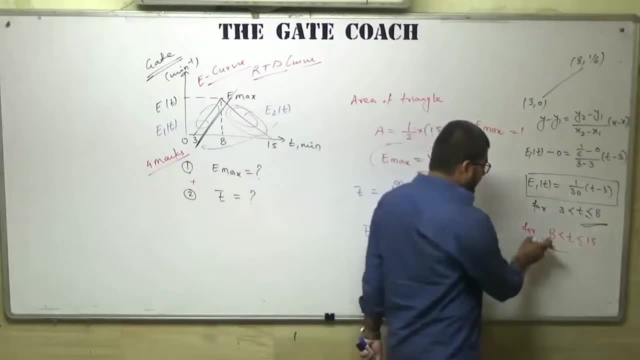 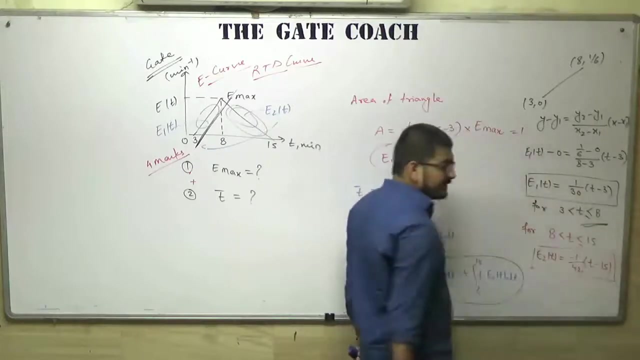 ok, and for time between 8 to, the function of e2 will come out like minus 1 by 42 t minus 15, which will be valid only for this time interval and when you put all those values of e1 and e2 in this equation.